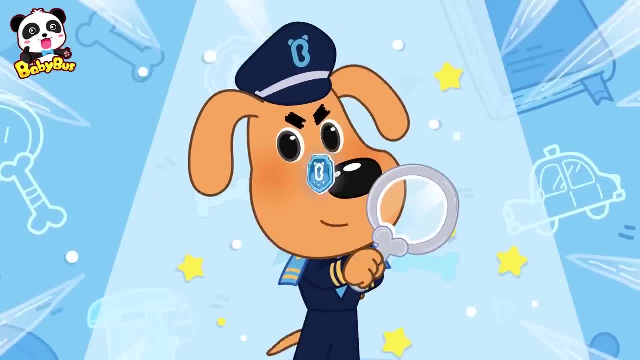 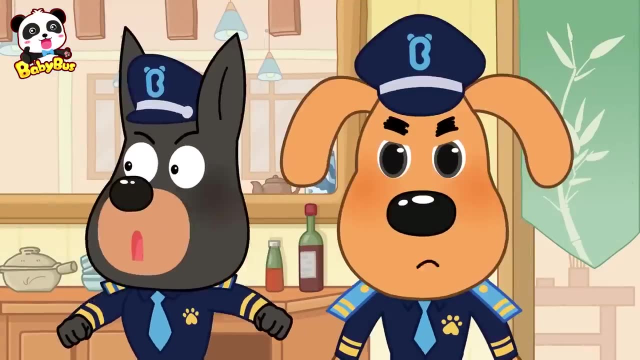 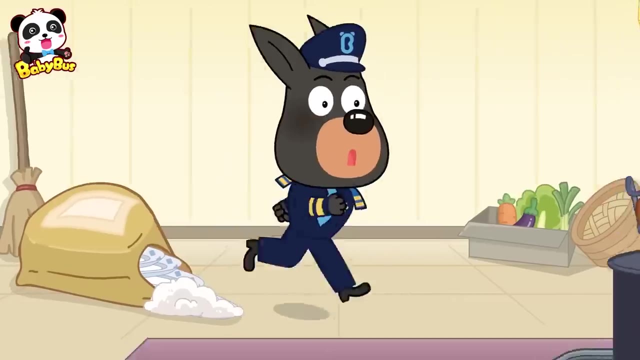 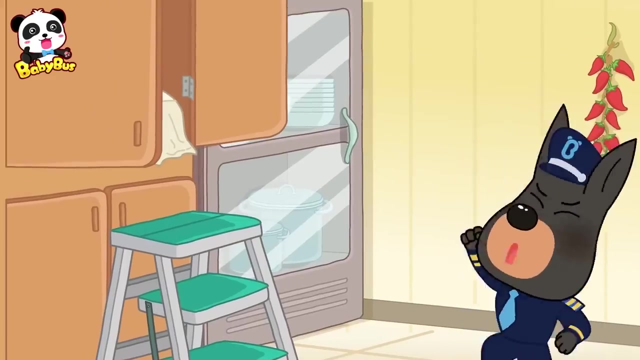 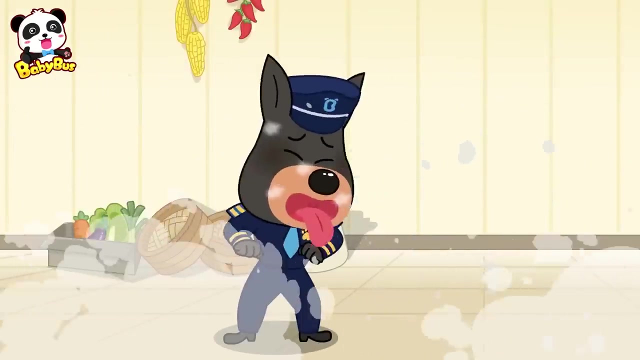 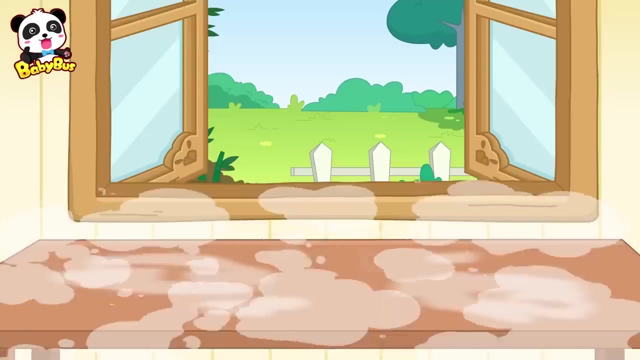 There's no case that I can't solve. If it was stolen, there must be clues left around here. Dobby, let's split up and look around. There's the thief. It's just flour. It's just flour Footprints. 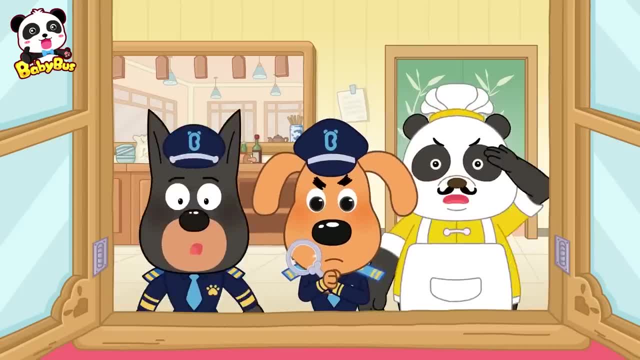 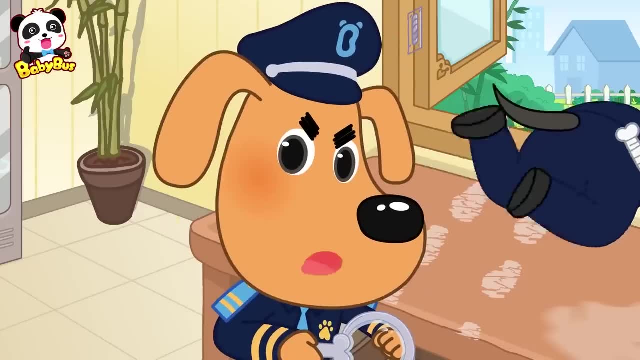 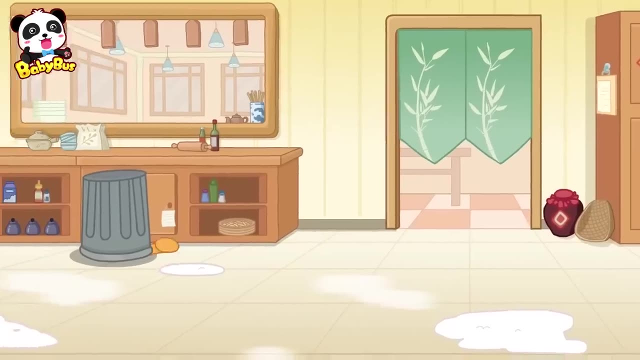 It looks like the thief broke in through the window. Unbelievable, I'm gonna catch the thief. Wait, The thief might still be here. What, What Look? There are no footprints leading out of here, So the thief must still be. 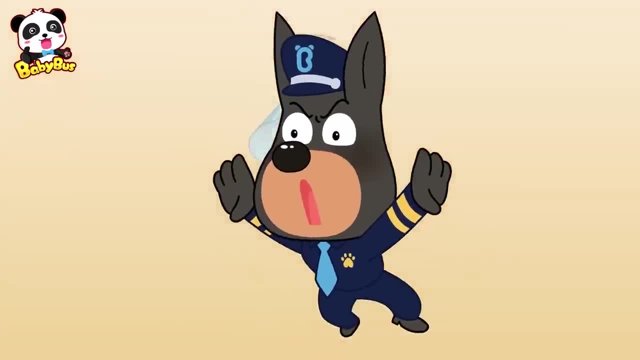 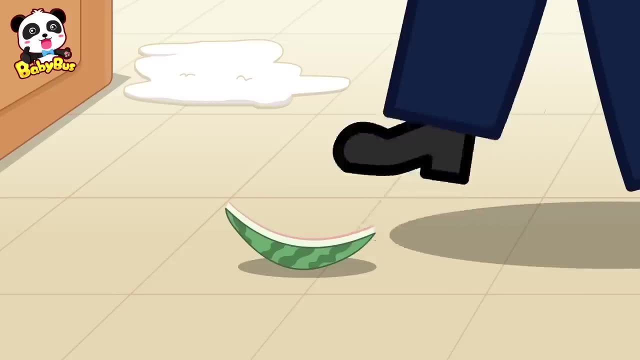 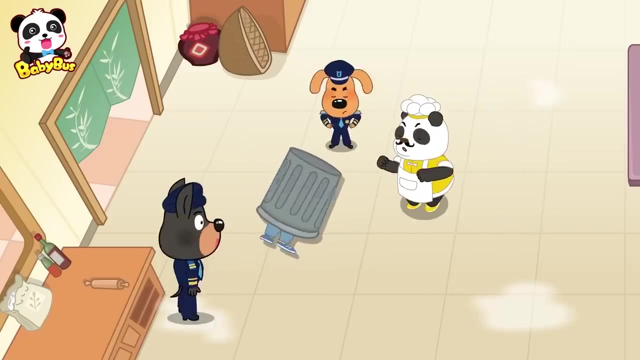 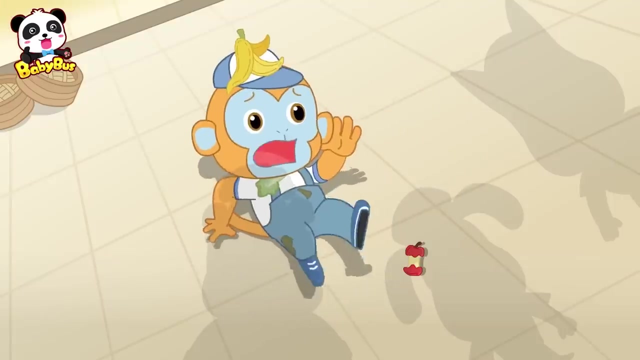 Here, You can't run away. I got you Ouch. Stop right there, Mr Monkey. It was you. No, no, it wasn't me. I'm sorry. I just wanted to see how the noodles are made. 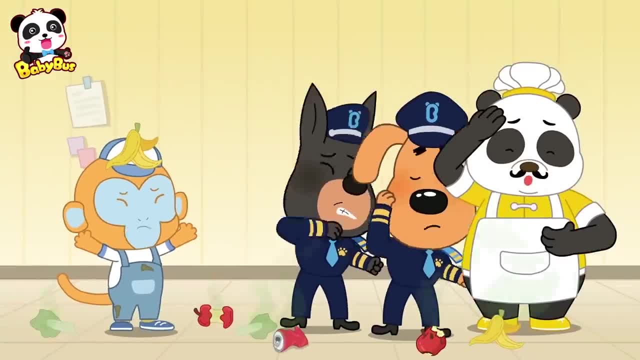 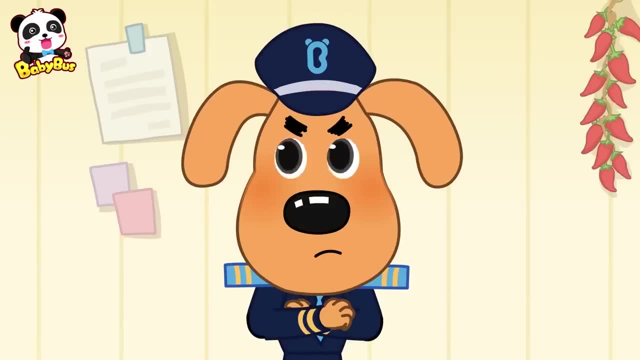 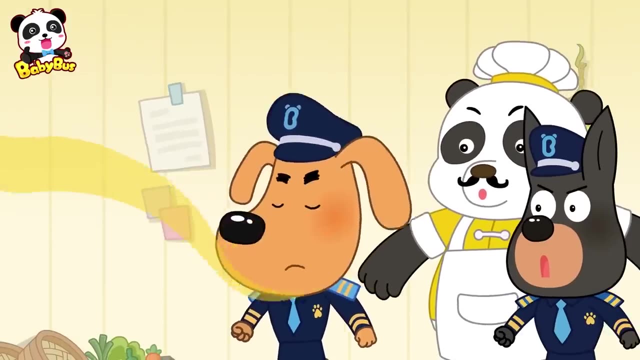 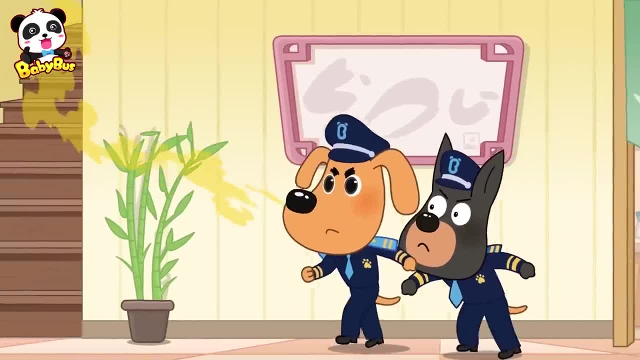 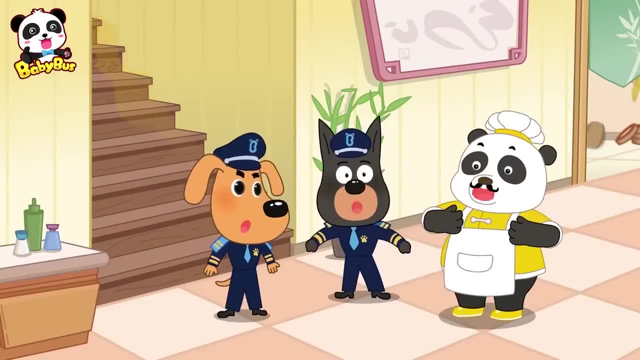 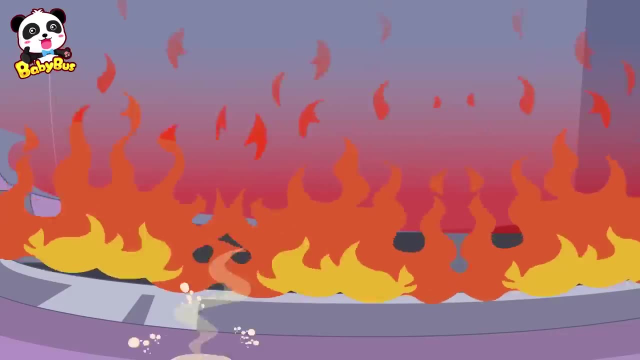 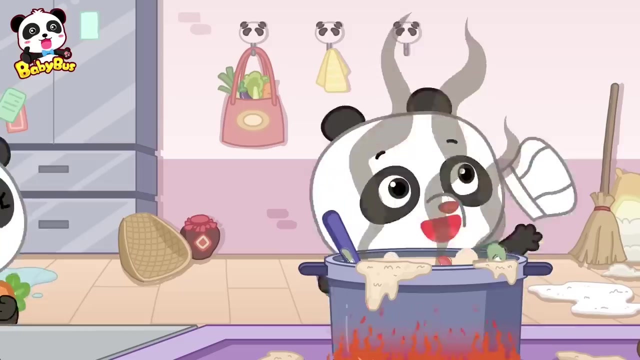 Oh, Oh, Oh, Oh, Oh Oh, The smell's coming from up there. There's another kitchen upstairs. Come on, let's go. Oh, Oh, Oh Oh. Tomato, Carrot, Mushroom, Cucumber. 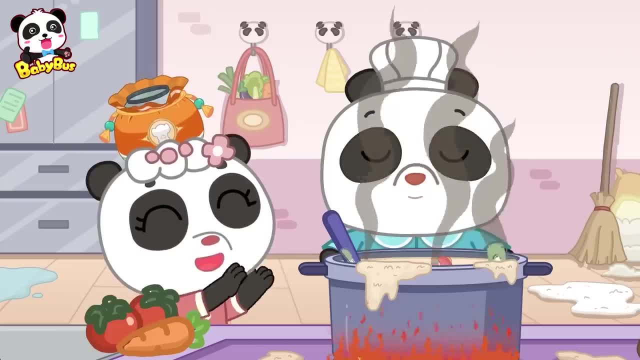 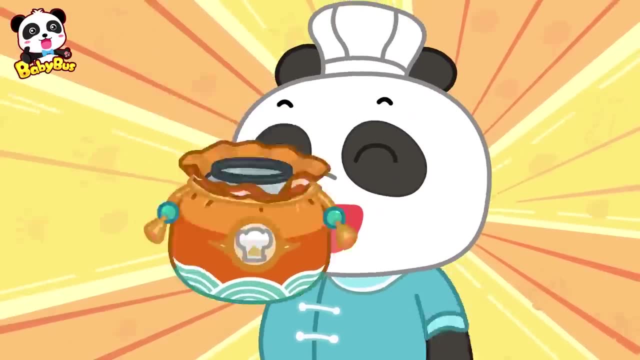 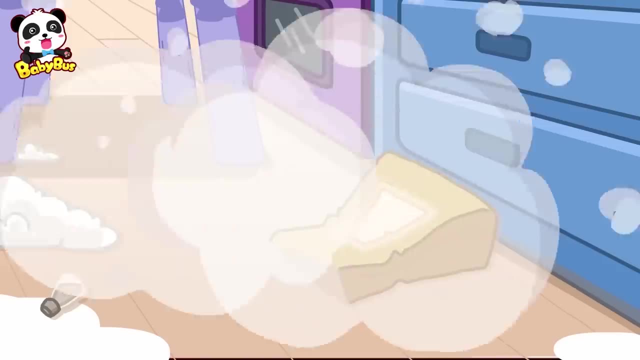 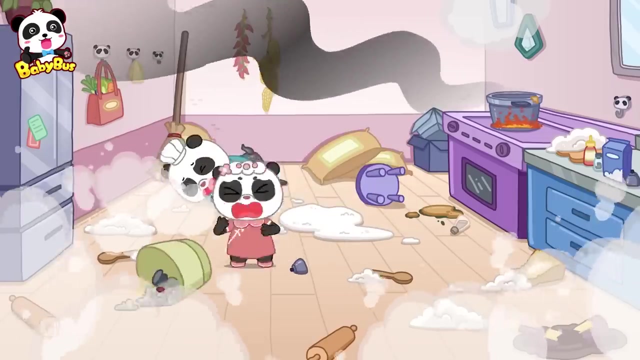 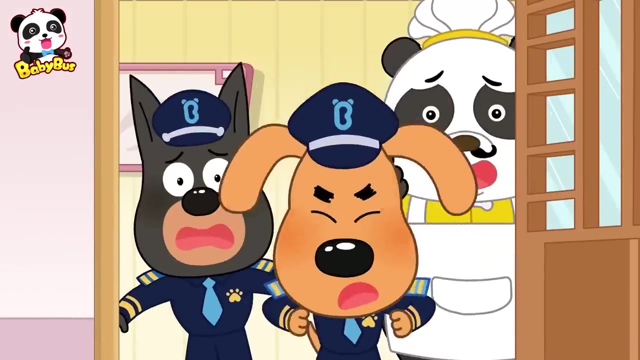 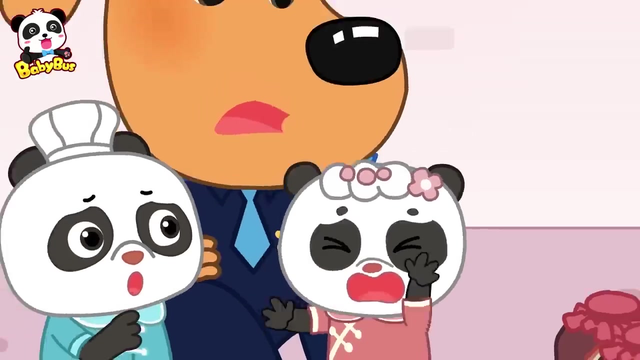 I'm the best chef in the world. Wow, Mister Chef, Sub* Red spice Here. Wow, Ow My eyes. It's my daughter. Hurry, Watch out My eyes. We need to send her to the hospital right now. 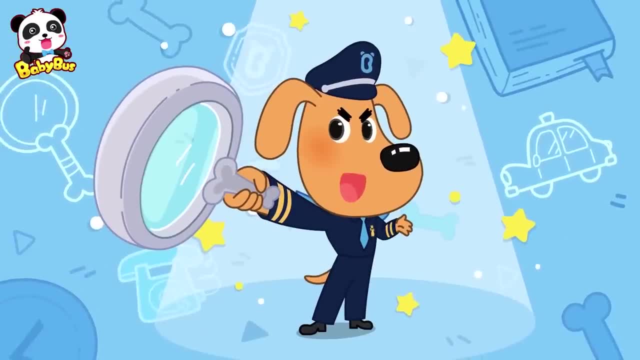 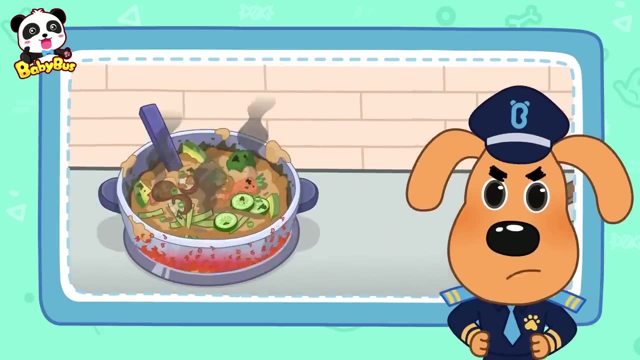 Sheriff Labrador's Safety Talk. Kids never play in the kitchen. There are sharp knives and tools, boiling water and electric appliances in the kitchen and they can hurt you Also. parents need to keep an eye on their children when they're in the kitchen too. 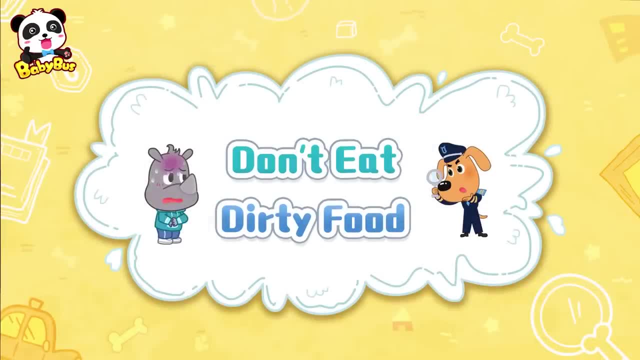 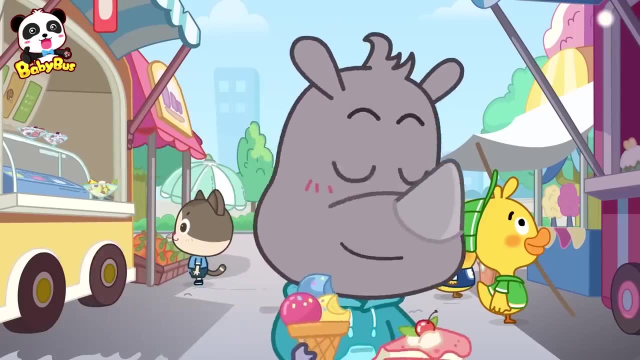 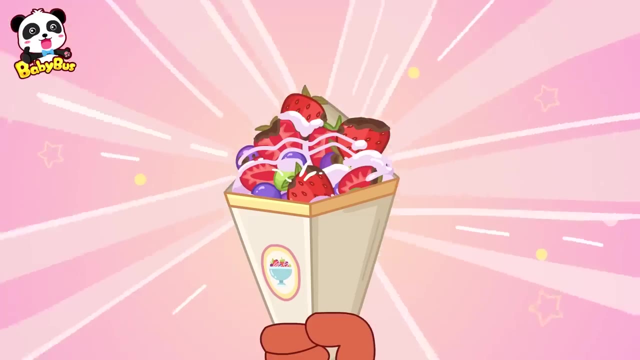 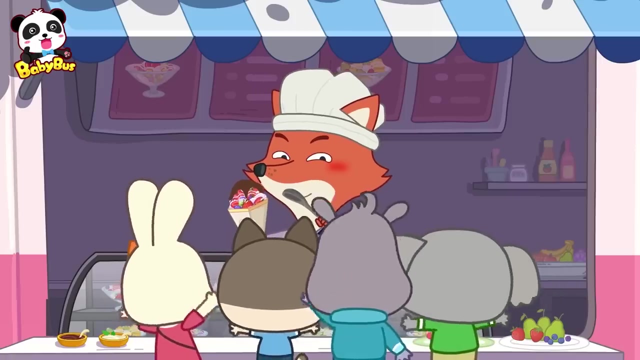 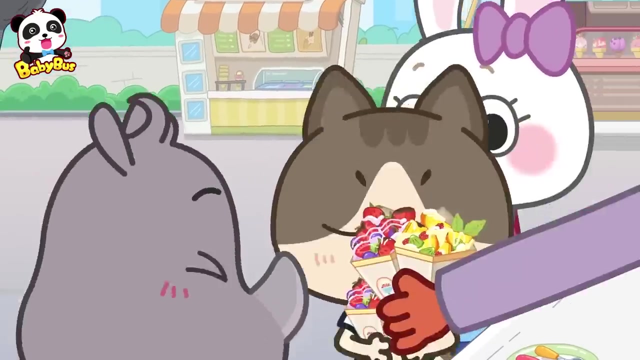 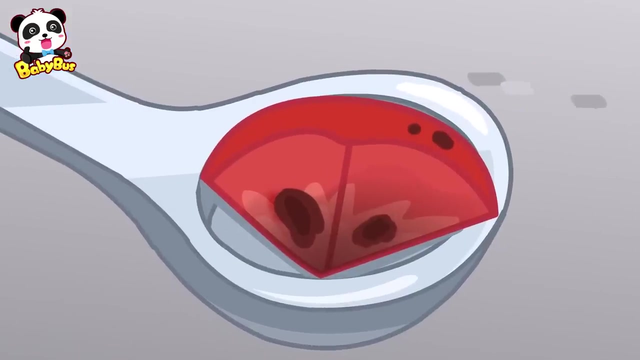 Woof, Don't eat dirty food. Wow, 滔, I want one, Mr Fox, I want one too. Alright, Just a moment Here. Here you are. What's this, Mr Fox? What's this black thing? 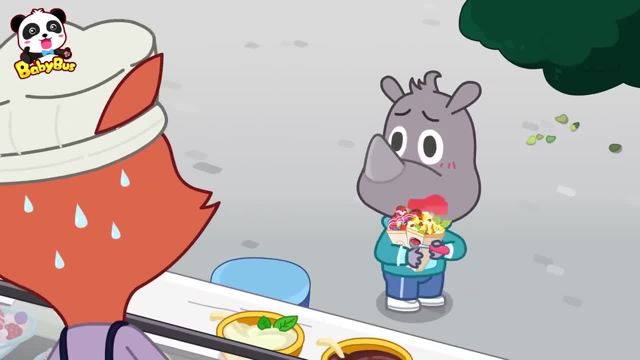 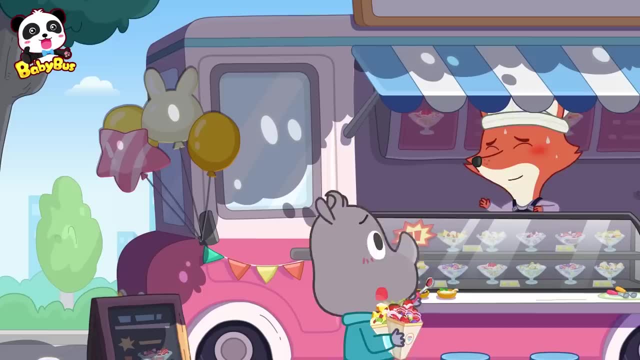 Uh, I don't know. It's a fake knife. You need to be careful. I don't want to hurt you. Be careful. Can't even cut, Can't you? Wellsure, It's just chocolate. You seem to really like my salad. I'll give you another one. 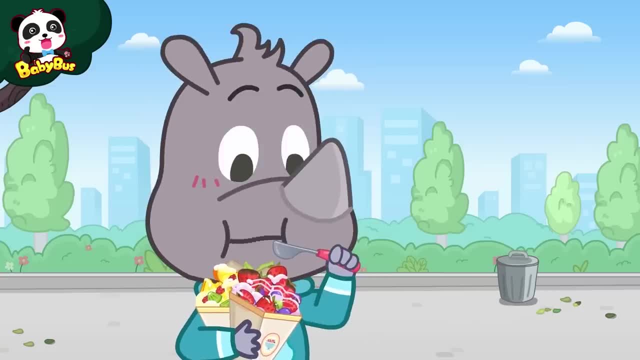 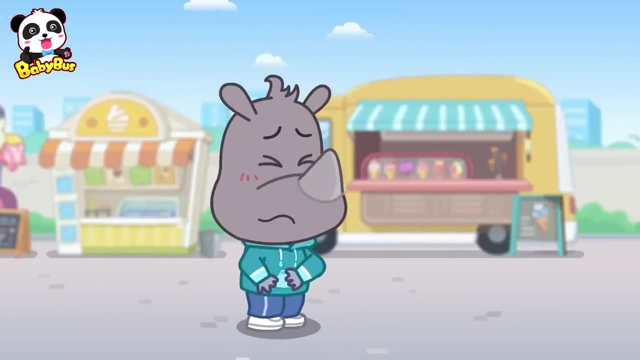 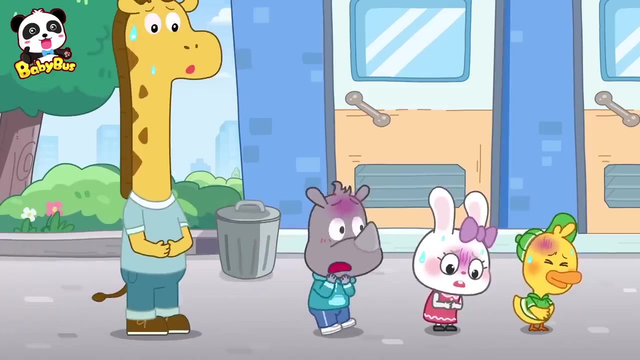 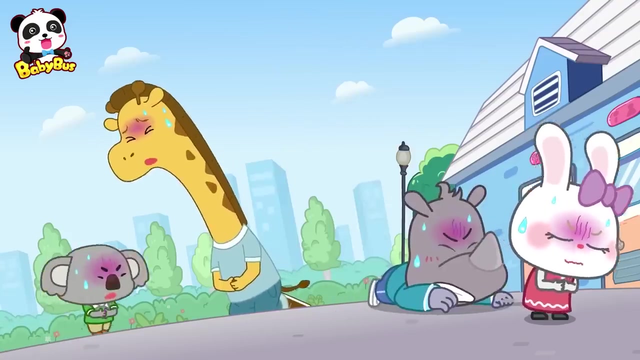 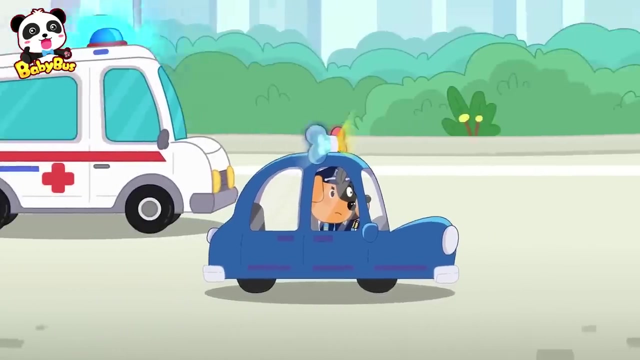 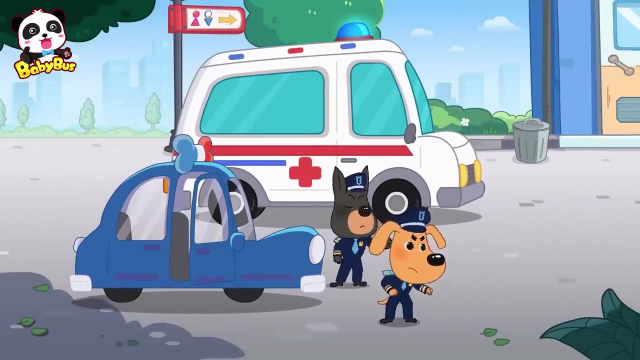 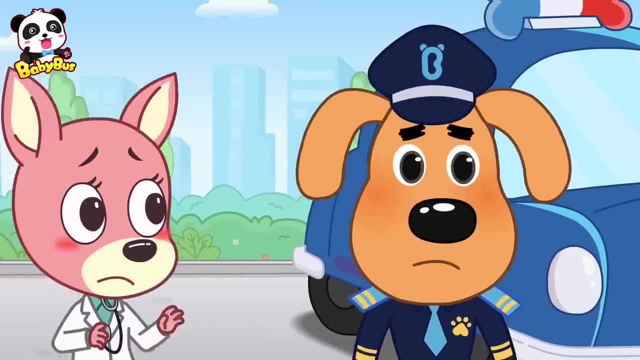 Thanks. Ow My tummy hurts. Ow Where's the restroom? Ah, Why are there so many people here? Ow My tummy, They don't look well. Ow My tummy, Sheriff Labrador. all these people got food poisoning. 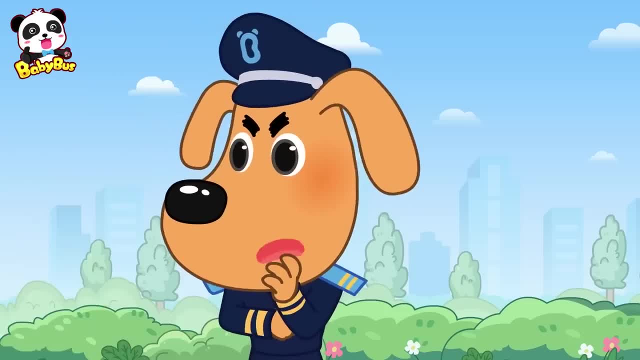 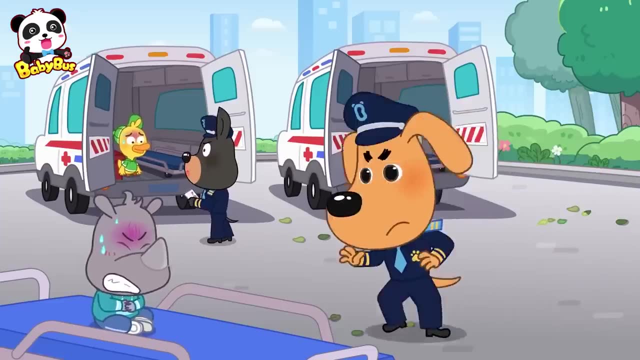 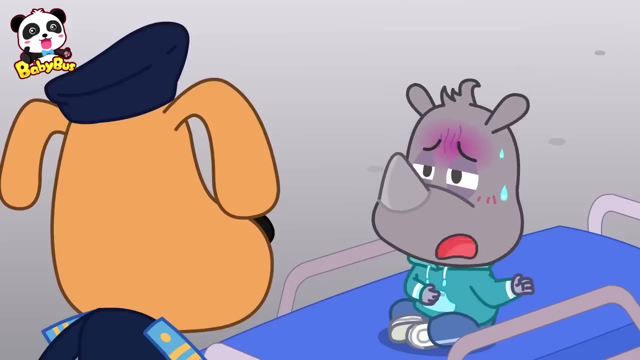 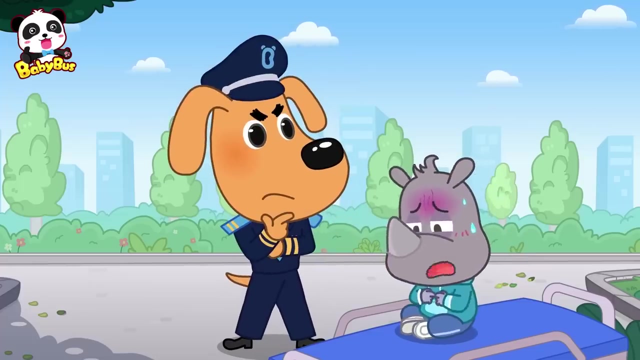 Something's wrong. Food poisoning Gobi. please find out what they ate today. Hey kid, How are you feeling? I've got the runs three times. Do you remember what you ate today? I had ice cream. I had ice cream, fruit salad and a cake. 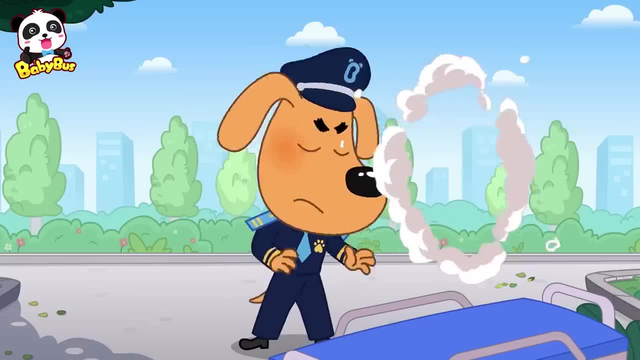 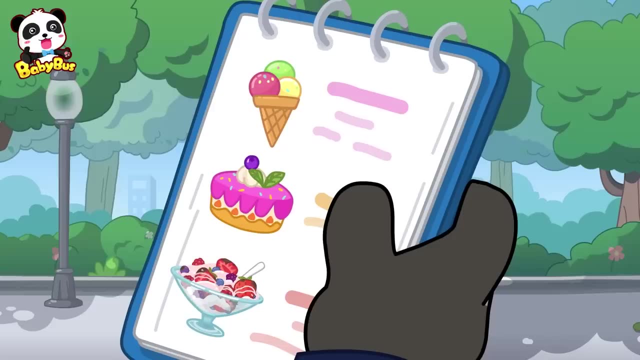 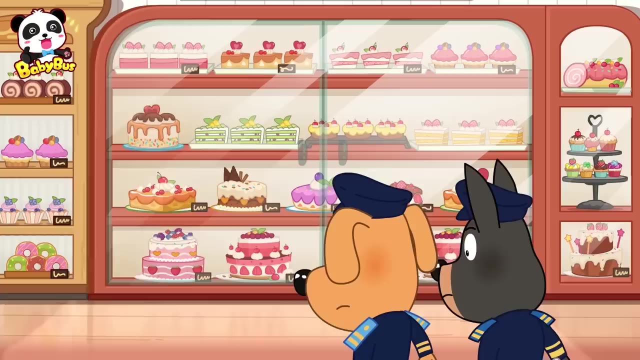 Oh no, I need to go again, Sir. here's the report. They all had ice cream, cake and fruit salad. Let's go investigate these shops. It's not me. My cake shop has been here for 100 years. 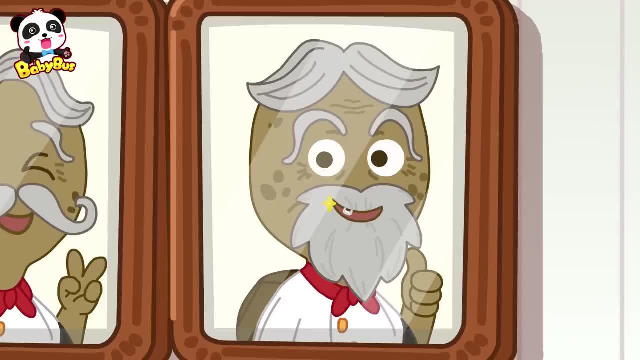 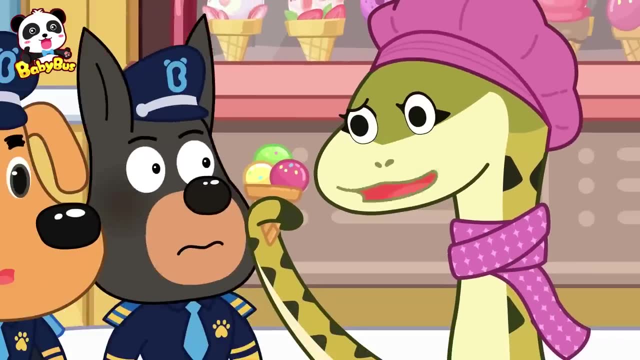 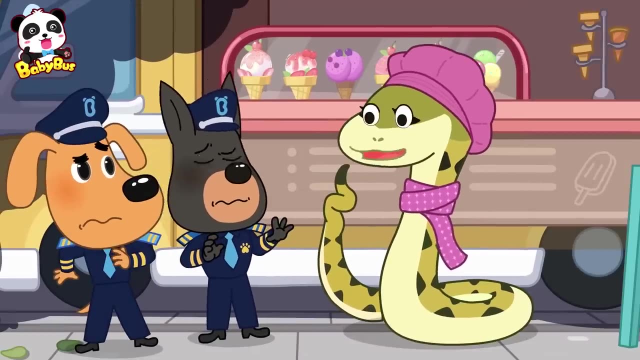 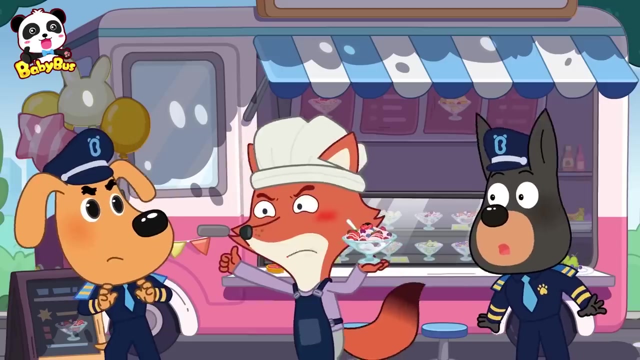 Such a thing has never happened before Since my grandfather's grandfather was here, Not me. I'm sure that nothing's wrong with my yummy ice cream. Look, My ice cream's fine. What Are you suspecting me? My shop is really clean. 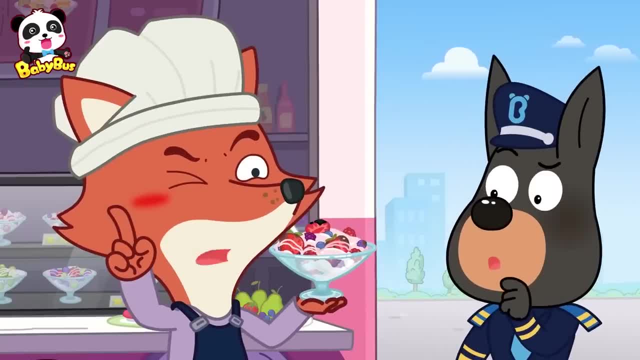 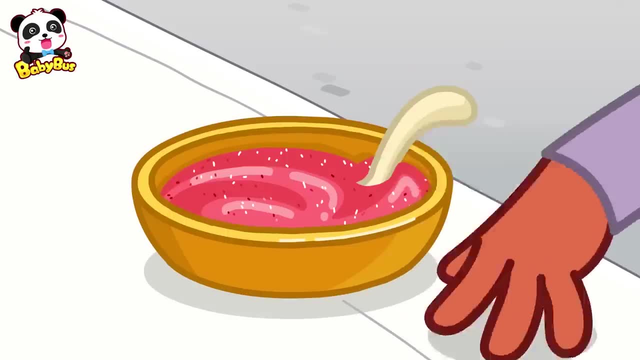 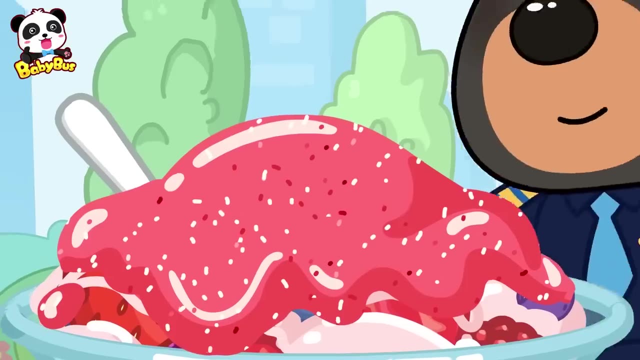 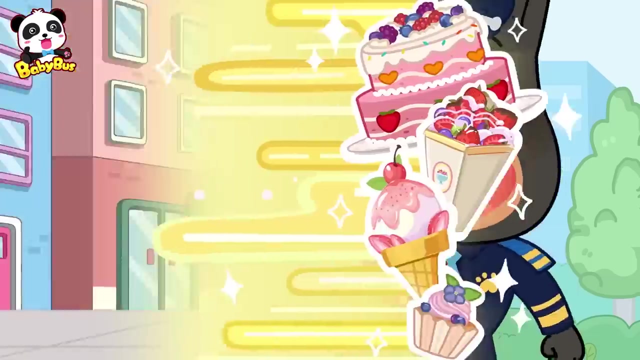 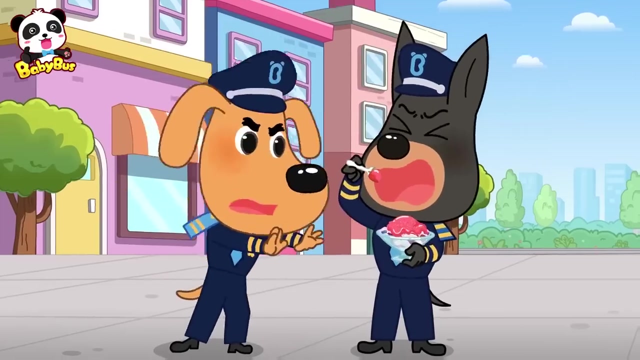 Every fruit salad is carefully selected by myself. I'm prepared by myself. Wow, I love fruit salad. I'd like to have one, please. Great choice. I don't think there is any problem with those shops. Don't eat it. 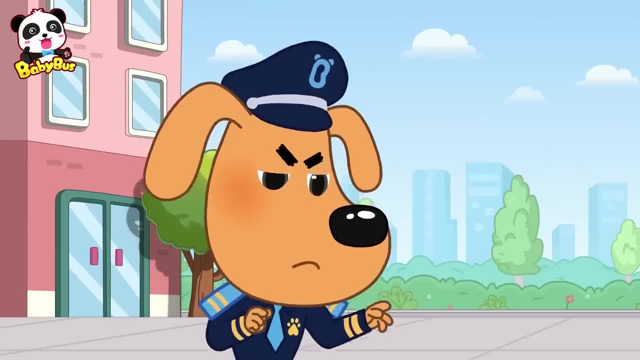 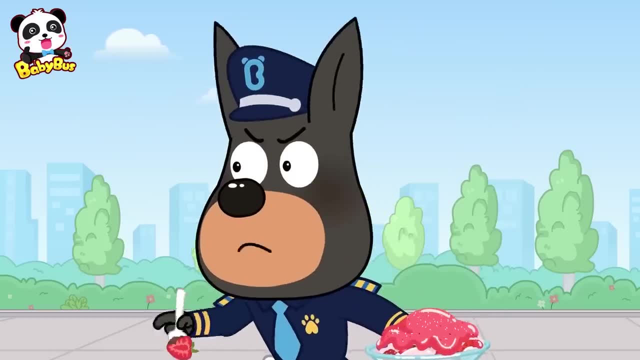 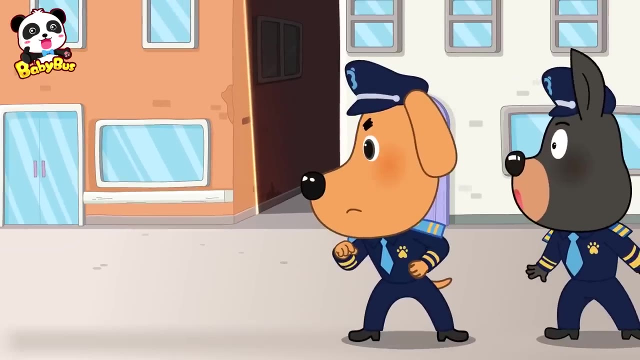 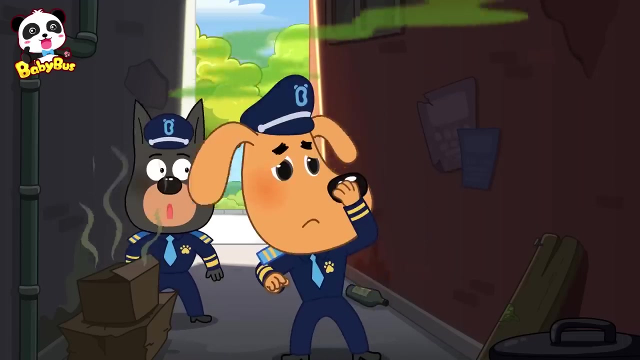 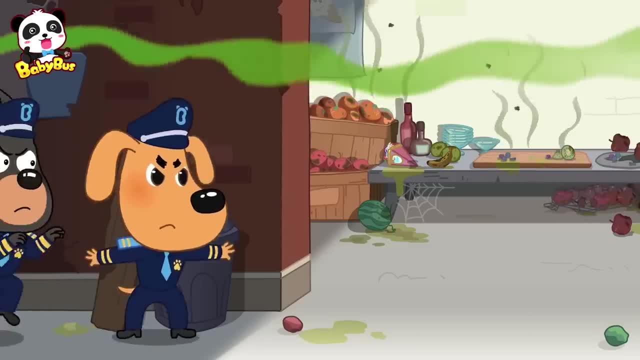 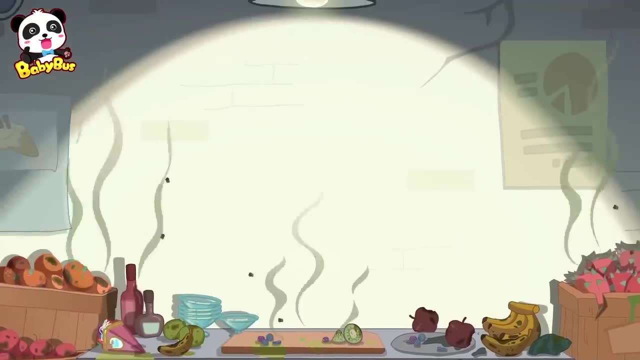 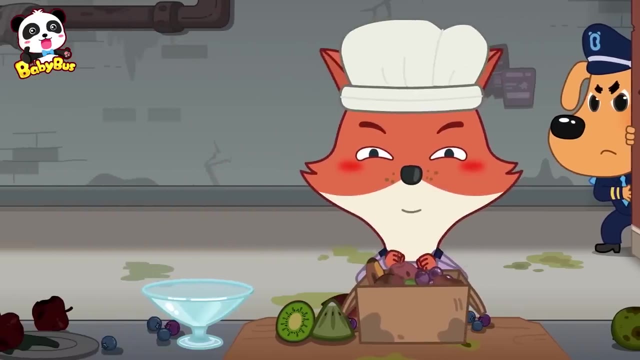 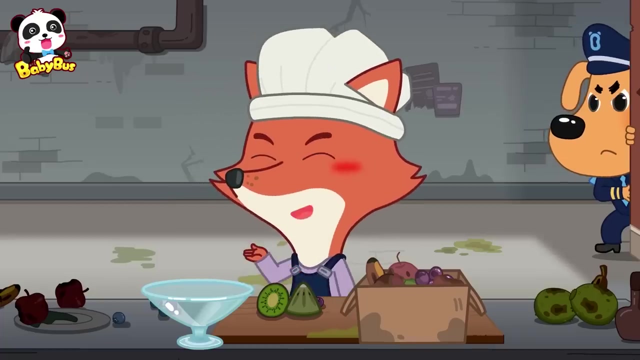 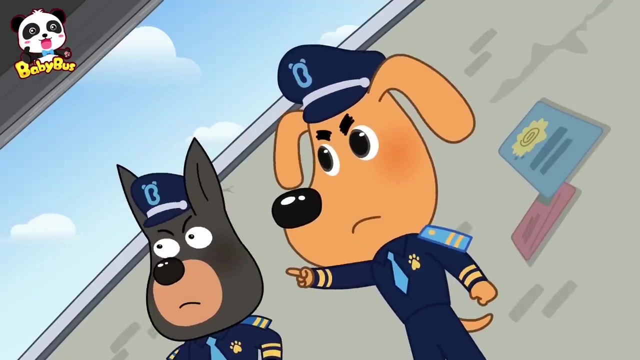 Let's go. Let's go. Rotten fruit is everywhere. Those police officers believed what I said. I don't care about rotten fruit, I'm not eating them anyway. Mr Fox, it was you who made people sick Police. 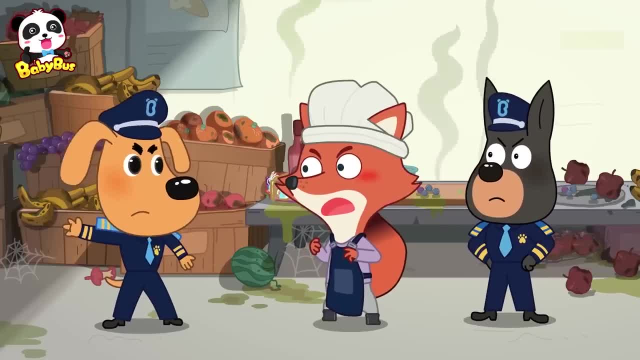 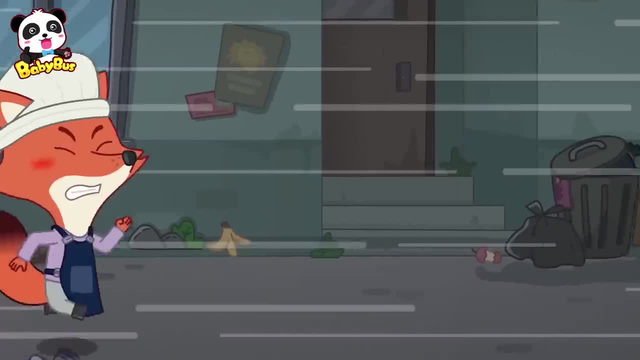 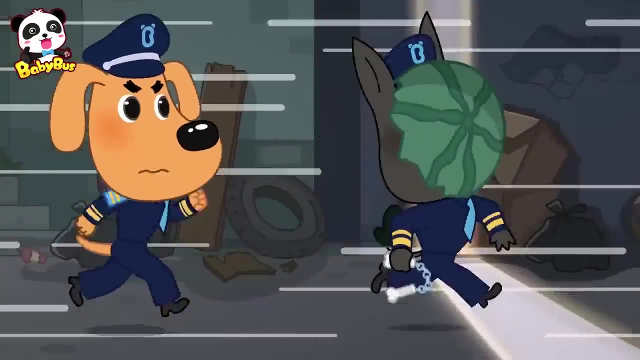 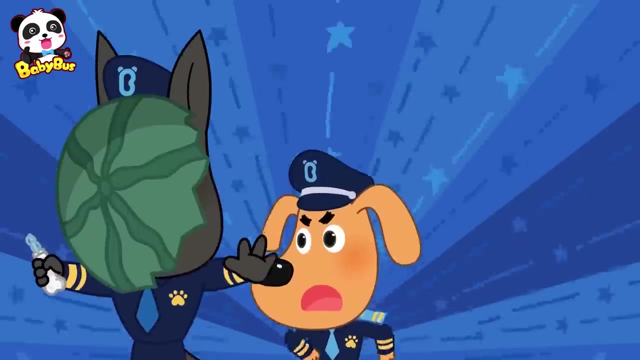 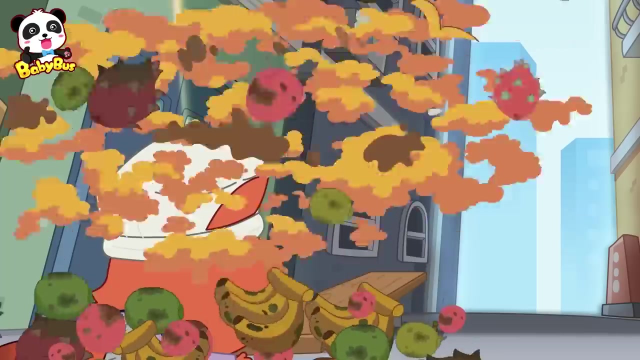 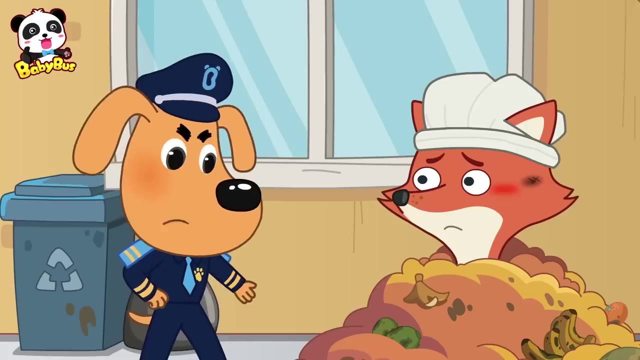 Come with us to the police station. Come with us to the police station. I'm going to run. I'm going to run. See you later, See you later, See you later. You can have it. It's so disgusting. You don't want to eat rotten fruit, do you? 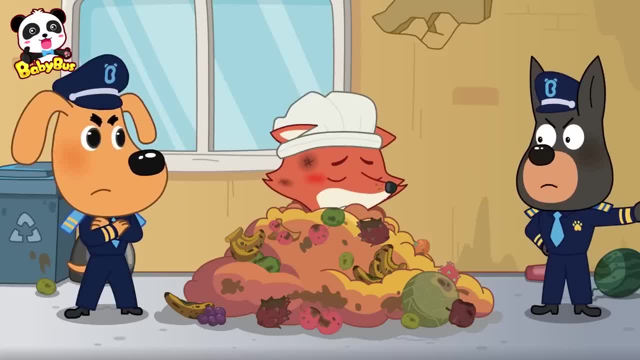 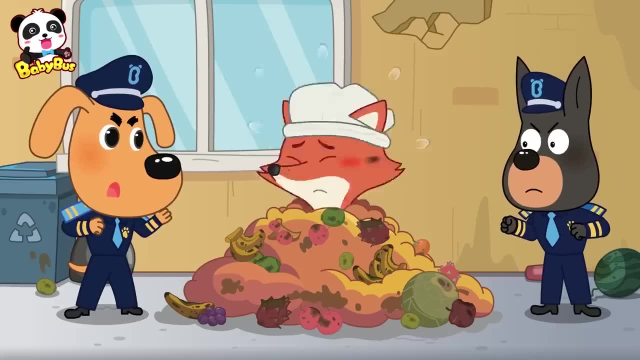 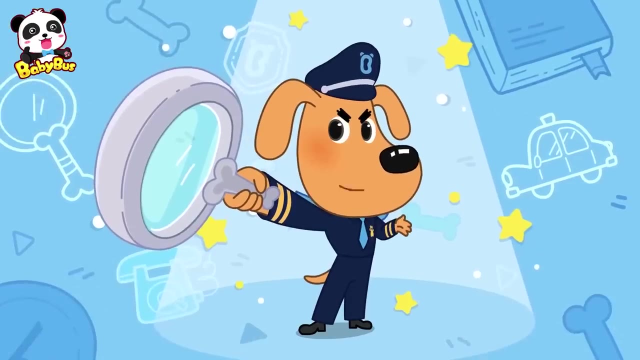 You don't want to eat rotten fruit, do you? You're so bad. You are going to the police station with us, My tummy. Please take me to the hospital first. Please take me to the hospital first. Sheriff Labrador's Safety Talk. 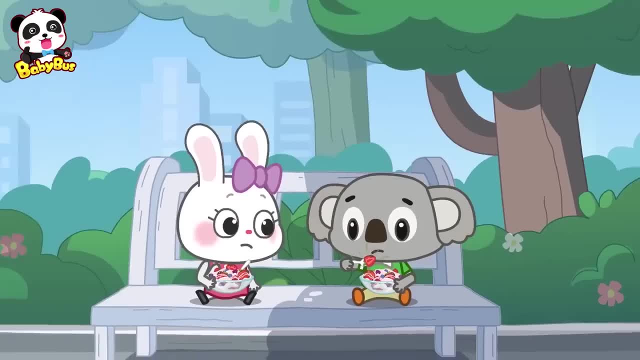 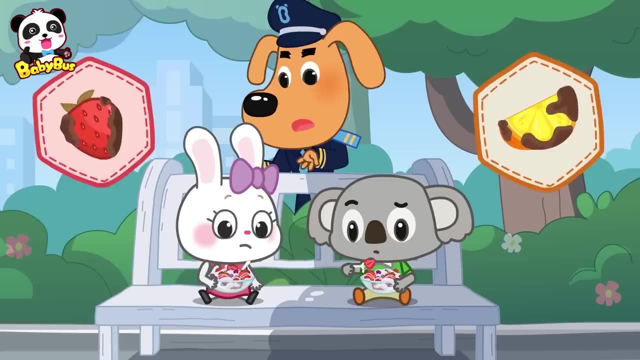 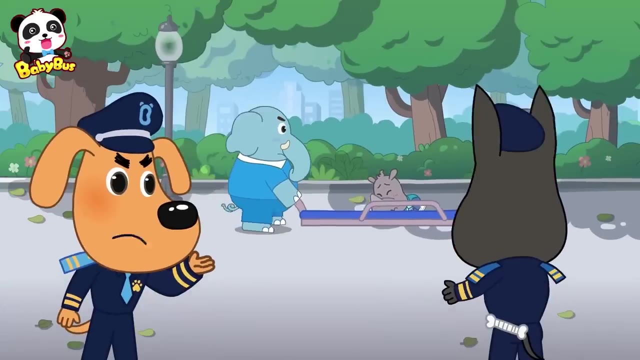 Sheriff Labrador's Safety Talk. Kids check your food before eating. Kids check your food before eating. If it looks dirty or rotten or it's past its expiration date, you shouldn't eat it. Rotten food can cause stomach ache and even food poisoning. 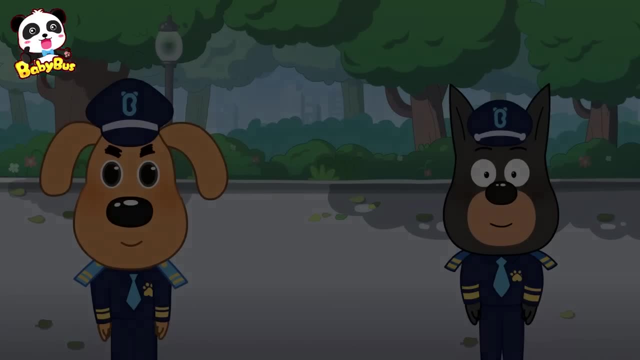 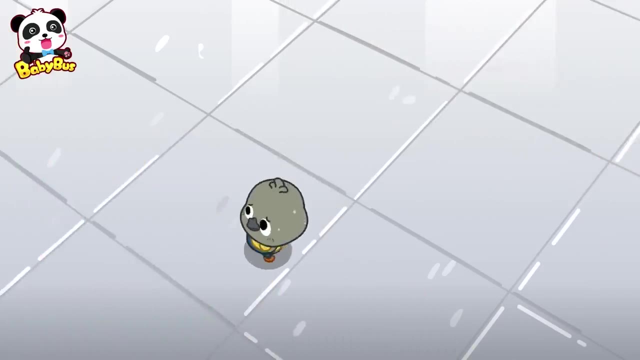 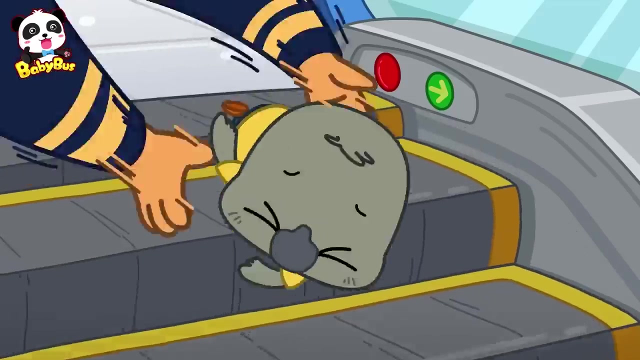 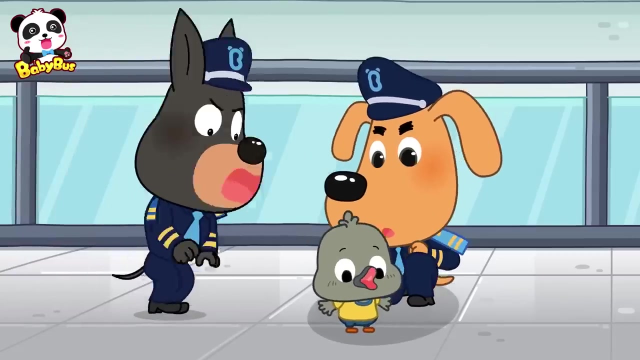 Please keep these in mind. Please keep these in mind. Baby swan got lost. Baby swan got lost. Mommy, Mommy, Ouch, Ouch, Ouch, Ouch, Ouch Ouch. Hey, little kid. 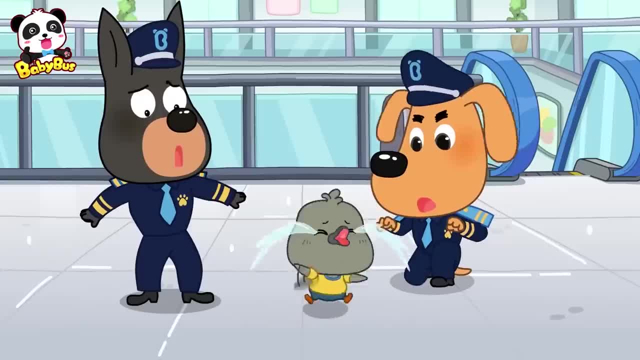 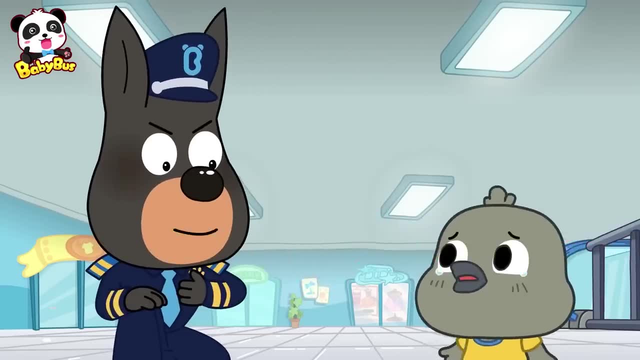 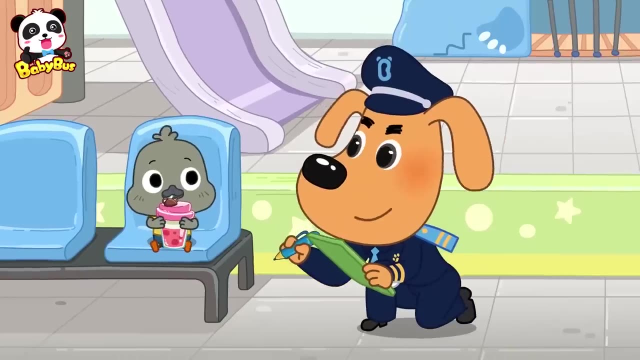 Are you alright? I lost my mommy. I lost my mommy. I lost my mommy. Don't cry, kid, Don't worry. There's no case that I can't solve. There's no case that I can't solve. There's no case that I can't solve. 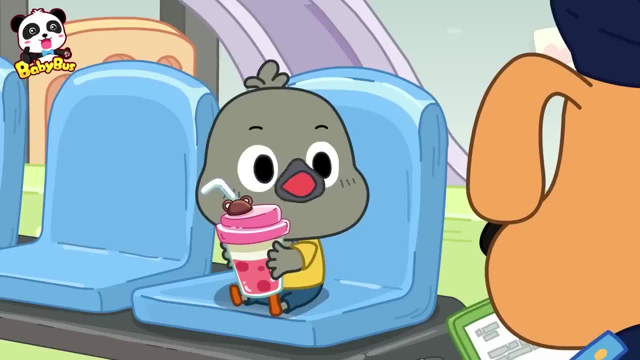 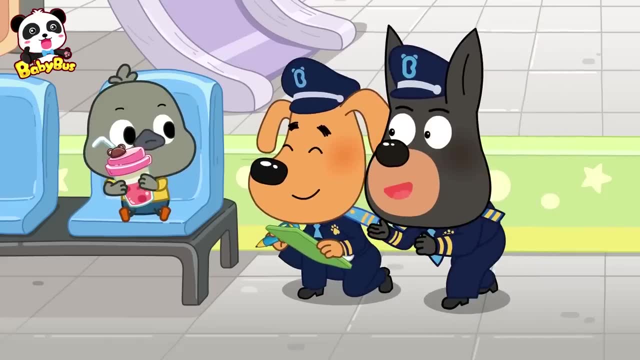 Kid, what's your name? My name is Gray And your mommy's name, Mommy. I mean, what's your mommy's name? I mean, what's your mommy's name? It's just Mommy, It's just Mommy. 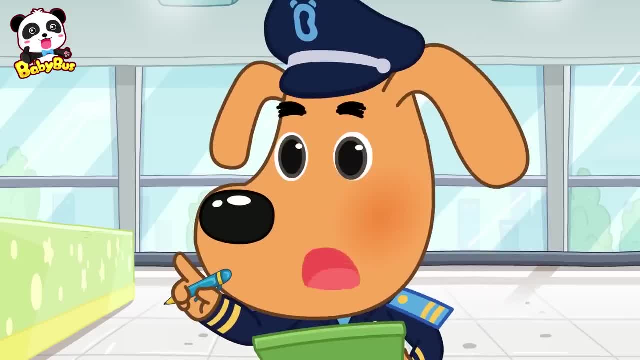 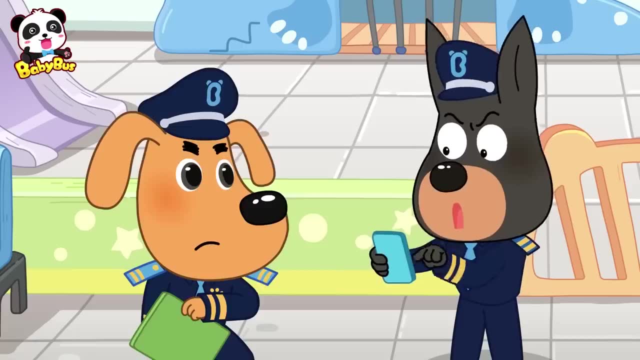 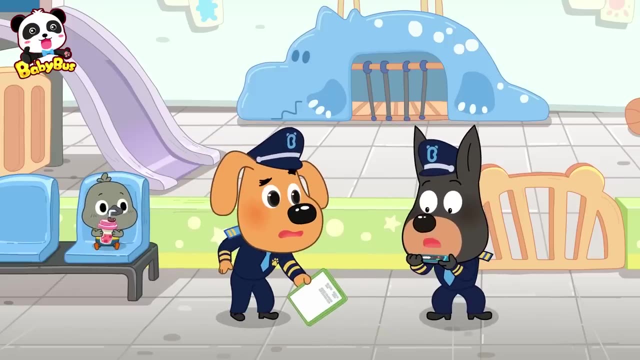 Well, do you know your mommy's phone number? Maybe 7773 and 3!. 7773 and 3!. 7773 and 3!. Hello, Hello, Hello. Are you Gray's mommy? Hello, Are you Gray's mommy? 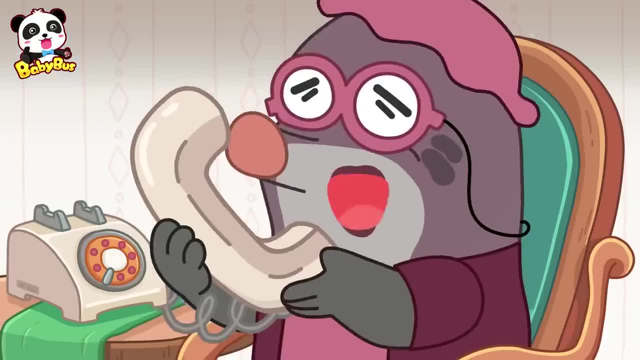 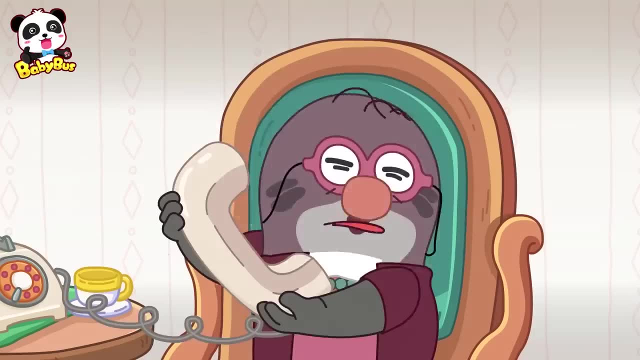 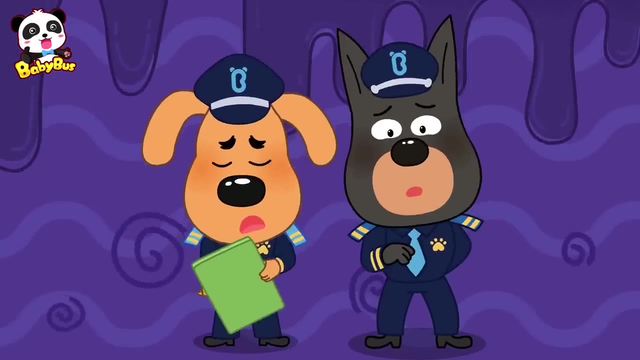 What Gray? What Gray Gray? Has my gray skirt arrived? Has my gray skirt arrived? It's not gray, Nothing, Sorry. Hey Gray, Are you sure it's 77733?? Hey Gray, Are you sure it's 77733?? 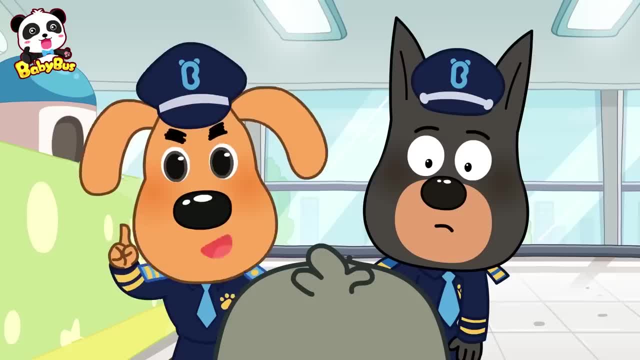 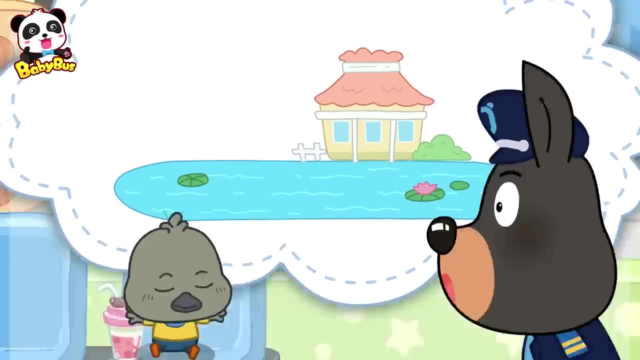 I don't remember. I don't remember. Then do you know your address? No, I just know there's a big pond by my house. I just know there's a big pond by my house, A pond. The wild goose family live by the pond. 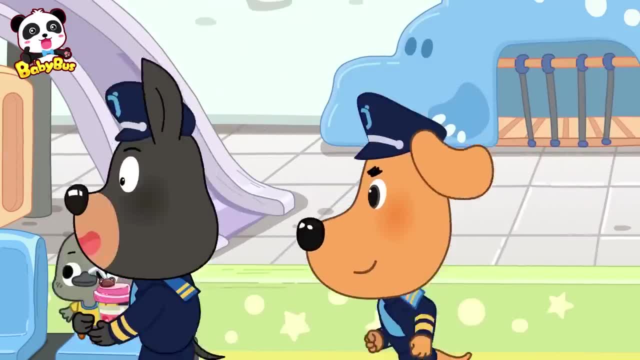 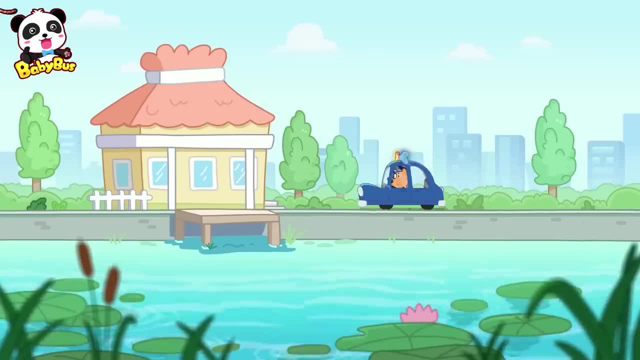 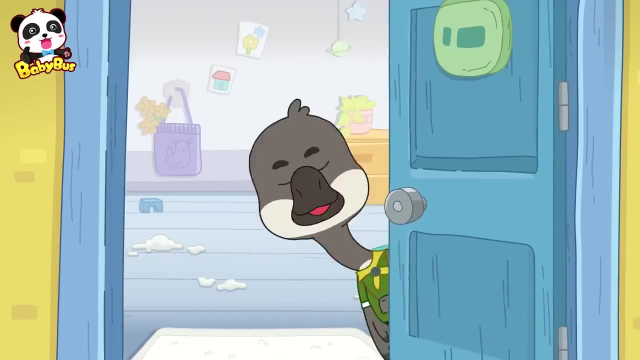 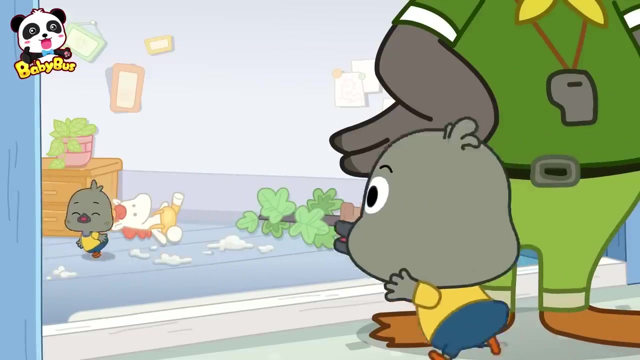 Great, Let's go to their house. Great, Let's go to their house. Great, Let's go to their house. A pond, What is that? Who is that? What is that? What is that? I want to see you. 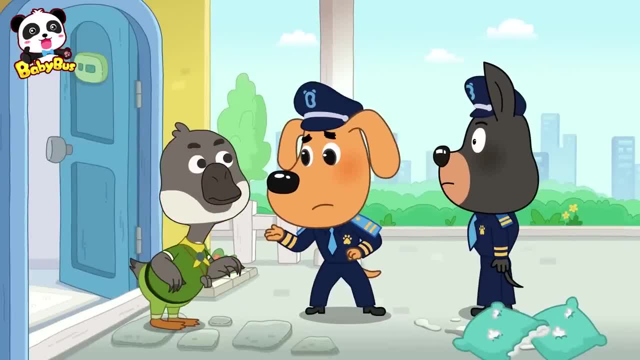 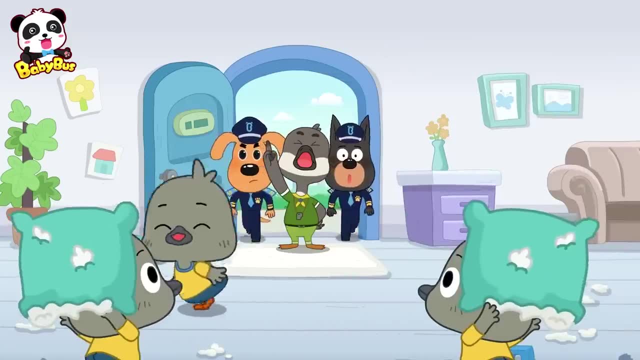 I want to see you, Sheriff Labrador, can I help you? Sheriff Labrador, can I help you? Mr Wild Goose, are all of your children home right now? Mr Wild Goose, are all of your children home right now? Gather up. 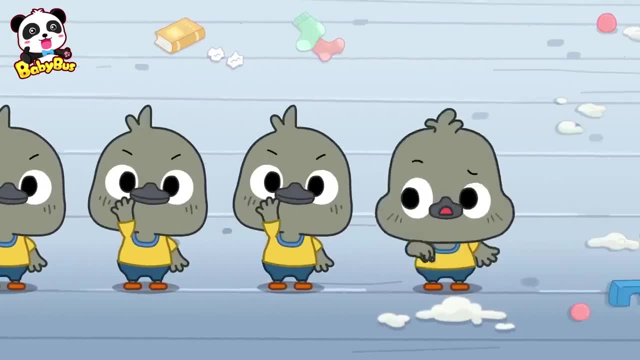 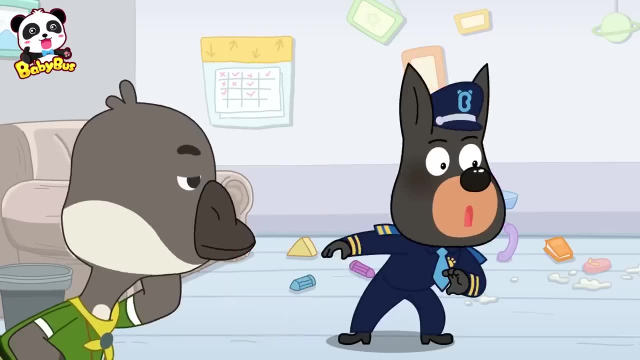 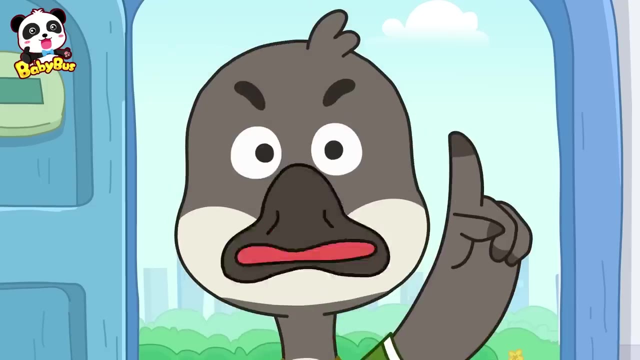 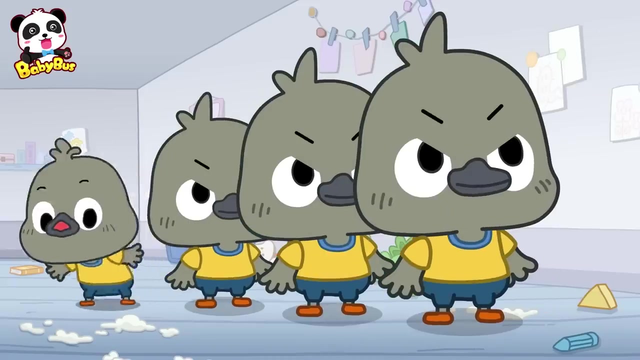 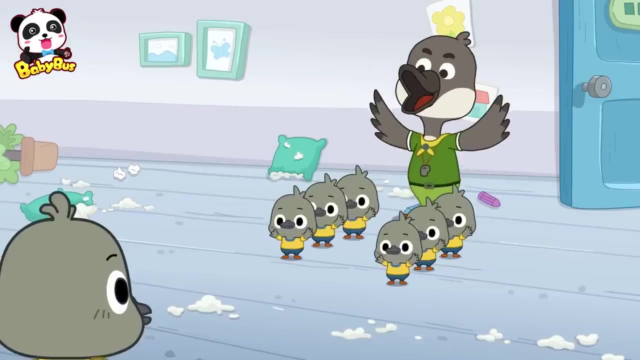 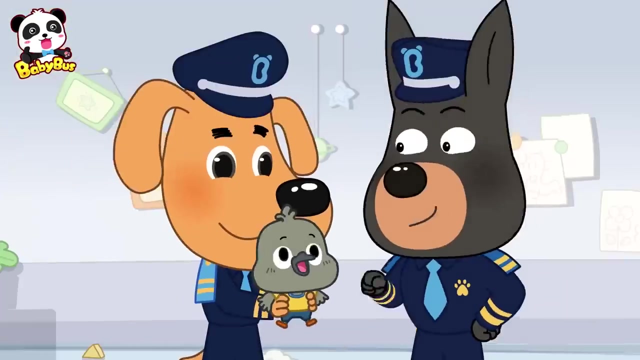 One, two, three, four, five, six, seven. I have only six children. Why are there seven? now? Where's Gray? Which one is Gray? Everyone line up. Wow, Wait, Aha, I got you Gray. 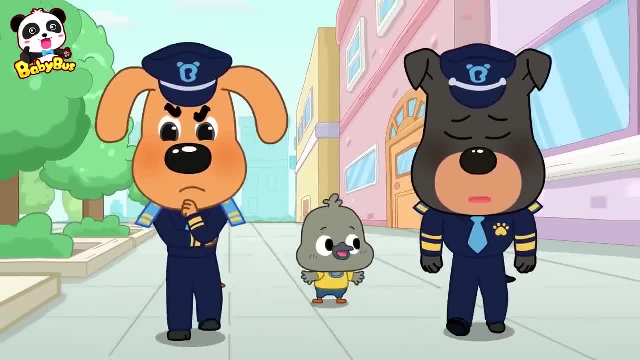 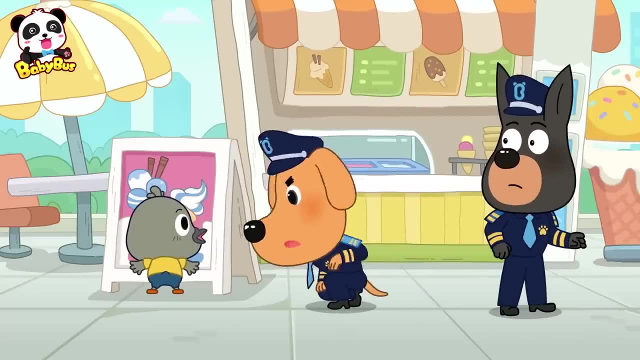 We haven't found any clue. Huh, Moomoo ice cream. I love Moomoo ice cream. Huh, Gray, do you and your mommy often come here to buy Moomoo ice cream? Uh-huh, Then let's go and ask. 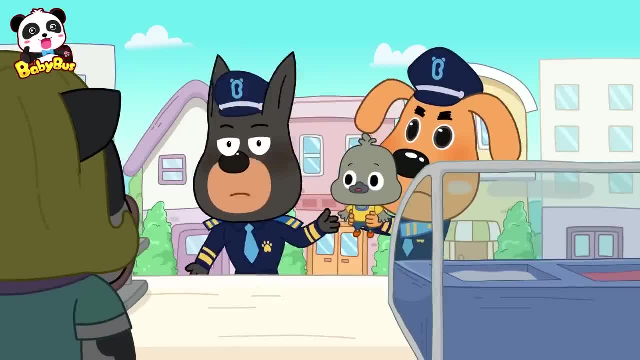 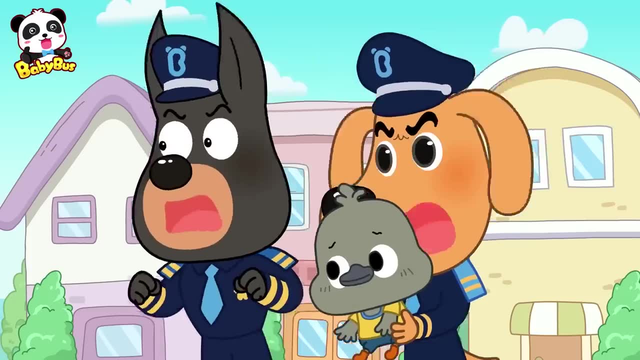 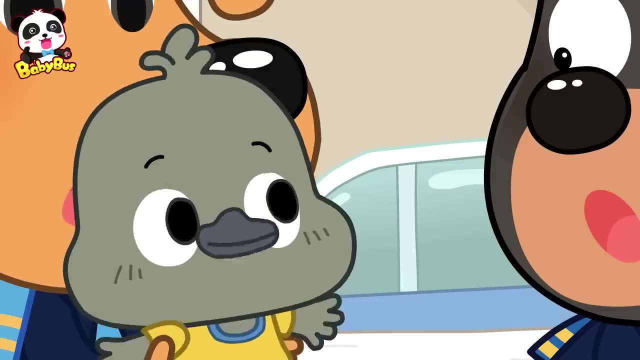 Hi, May I help you, Mizka? Do you know Gray here? Gray, What are you doing here? Your mommy was looking for you. Where did she go That way? Huh, Mommy, A swan. So Gray is a little swan. 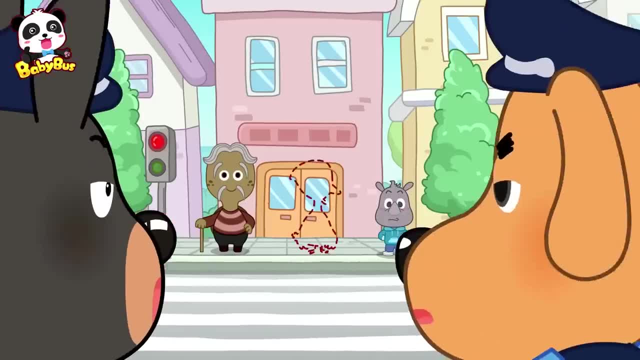 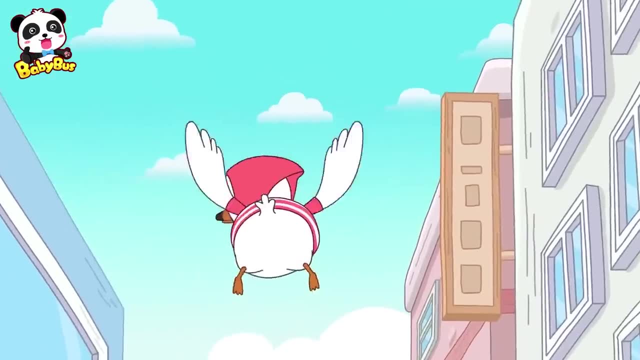 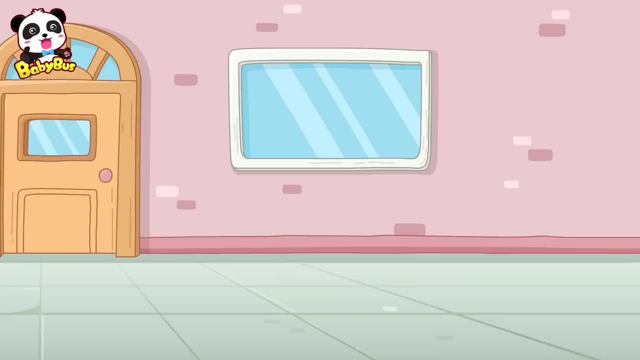 Mommy, Mommy, Mommy is missing. She's over there. Where's my child? Oh, Coming through. Sorry, Excuse me, We can't catch up with her. What do we do? Huh, Huh, Huh. 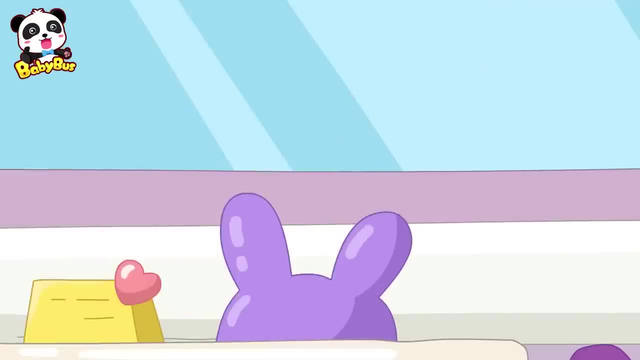 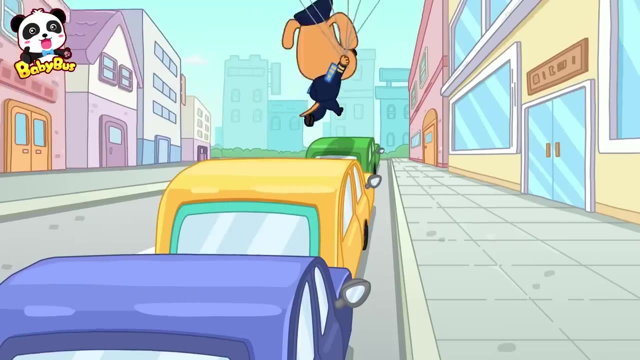 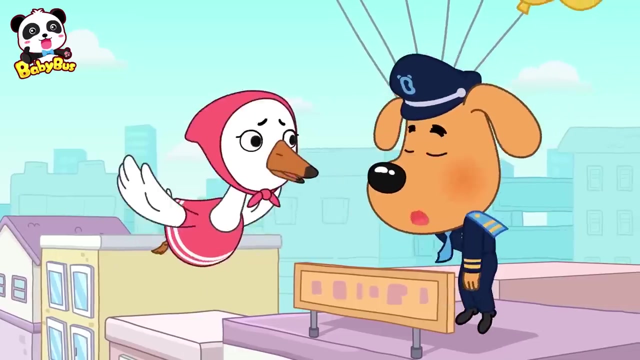 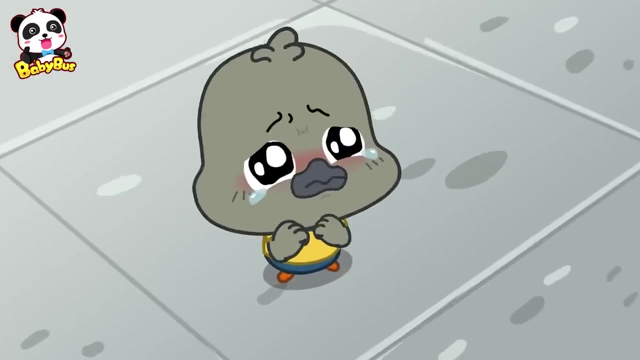 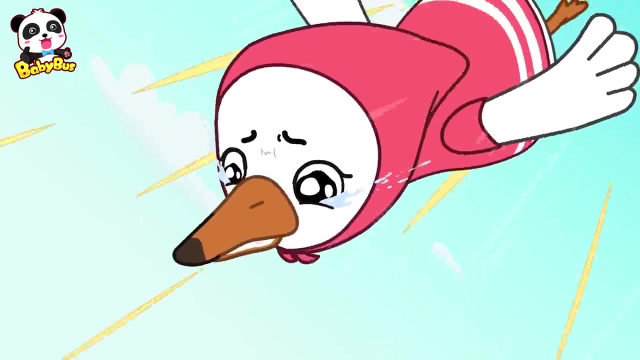 I have an idea, I have got a big idea. Miss Swan, Miss Swan, Sheriff Labrador, Finally, Look over there. Mommy, Uh, Mommy… Um… Mommy… Mommy… Oh, sweetie, Oh, where did you go, my child? 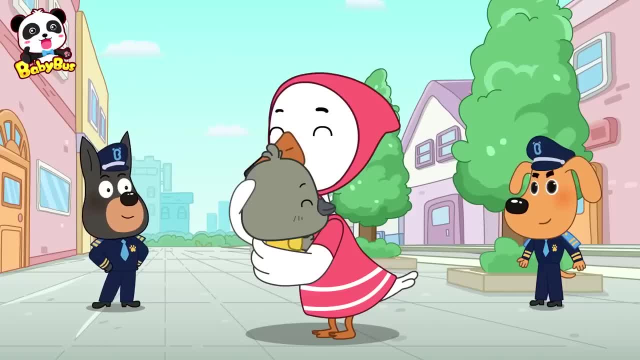 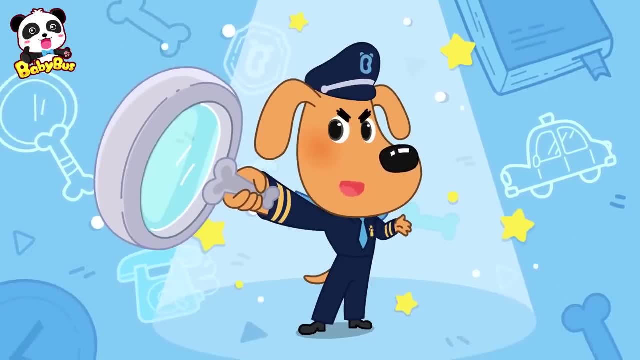 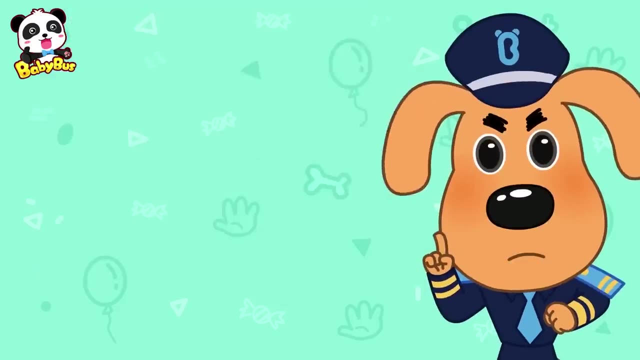 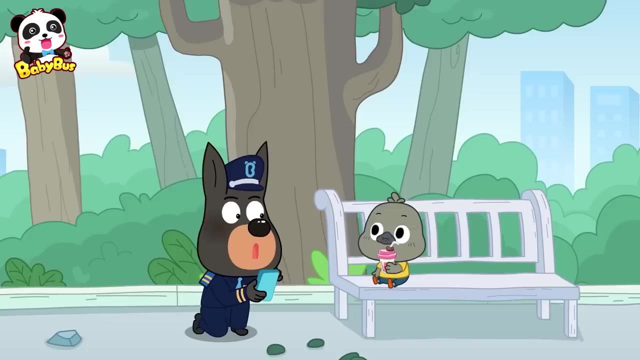 Oh, I've been so worried about you. Sheriff Labrador's Safety Talk. Kids, when you go out with your parents, you should always stay close to them And if you lose them, stay where you are and wait for them Or ask a police officer for help. 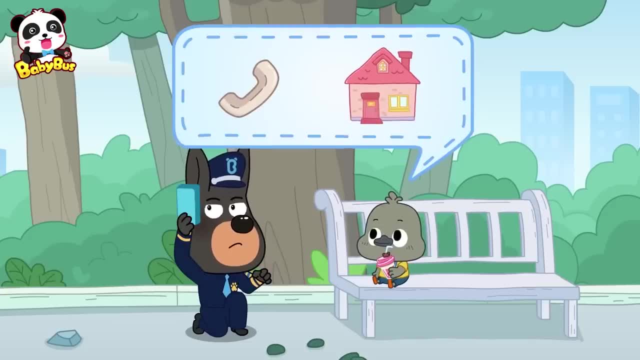 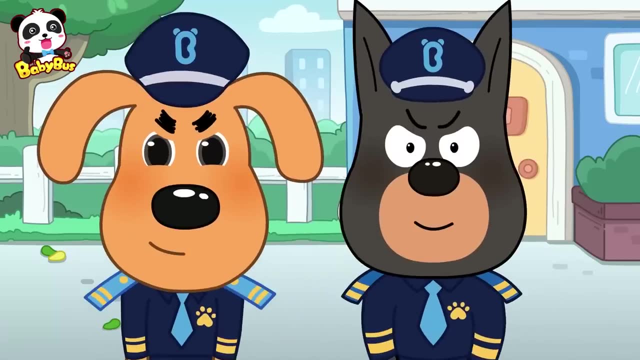 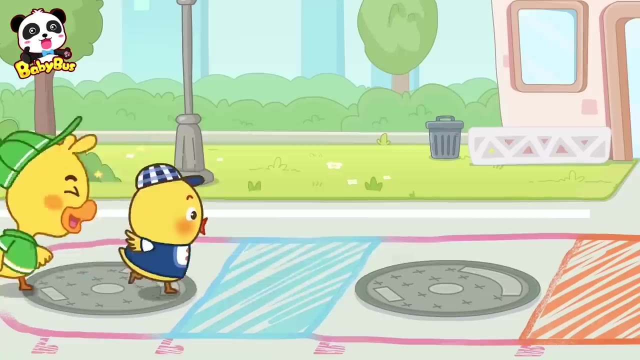 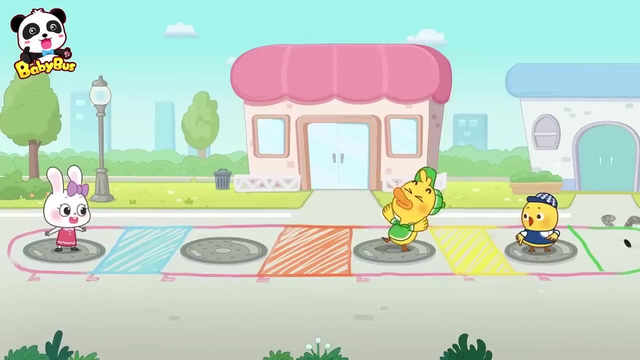 Also make sure to memorize your parents' phone numbers and your home address. It will help police officers find your parents. Please keep these in mind. The Dangerous Manhole Cover Three little children Jumping and having fun. Hello, hello, Where are you? 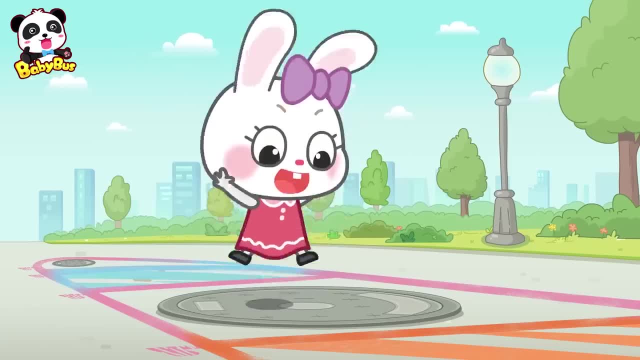 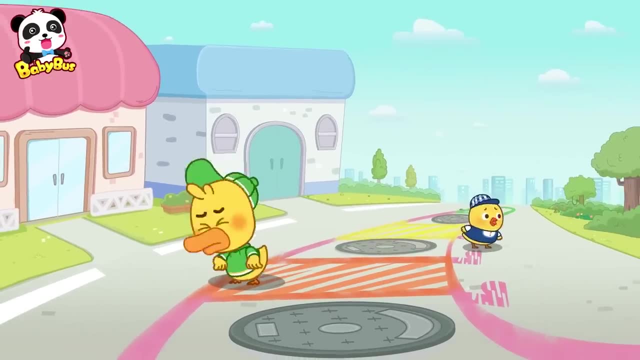 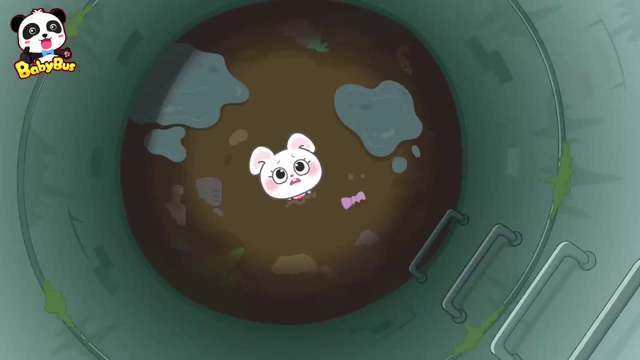 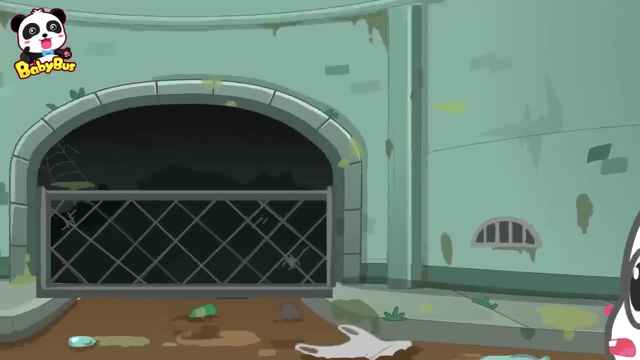 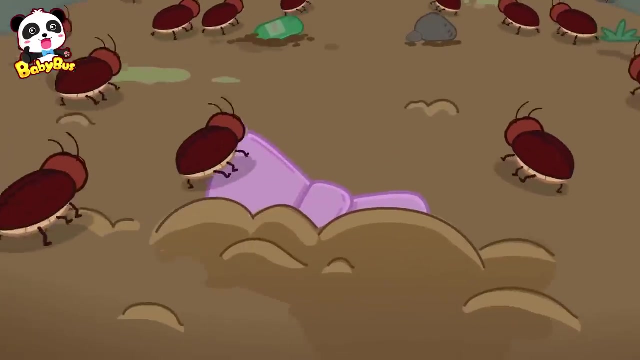 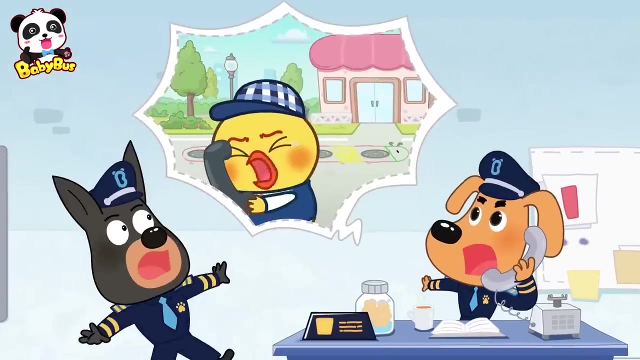 I, I, I, I'm Little Rabbit. Little Rabbit, Where are you? Ow, Ow, It hurts, Woof. Hi, I'm Sheriff Labrador. Sheriff Labrador, Little Rabbit, is missing. We can't find her anywhere. 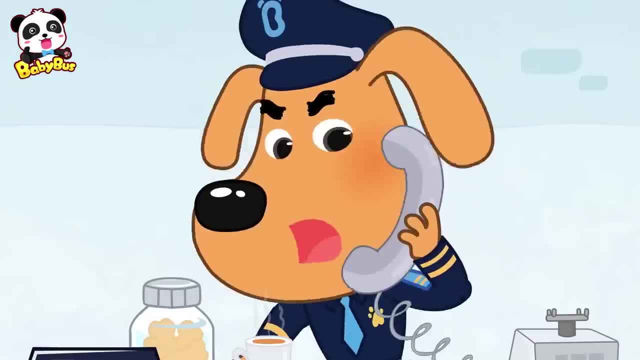 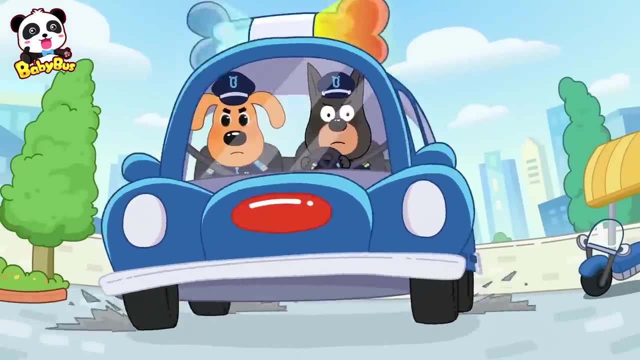 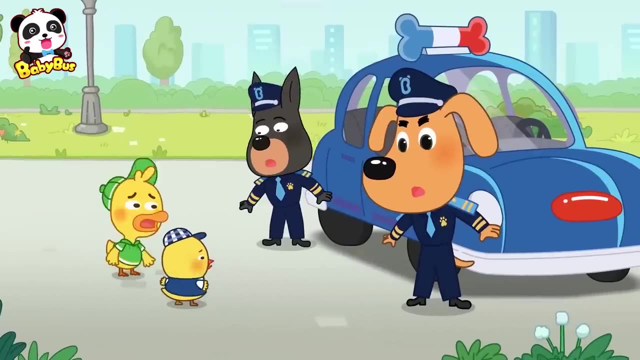 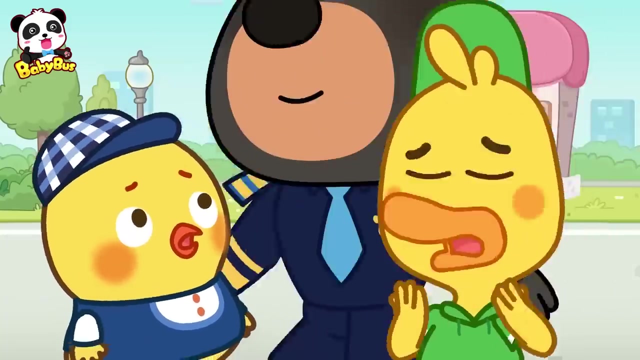 Please come help us. Don't worry, kids, We'll be right there. Woof, Woof, Sheriff Labrador. we were playing with Little Rabbit here and suddenly she disappeared. I'm so scared. Don't worry, we'll find Little Rabbit. 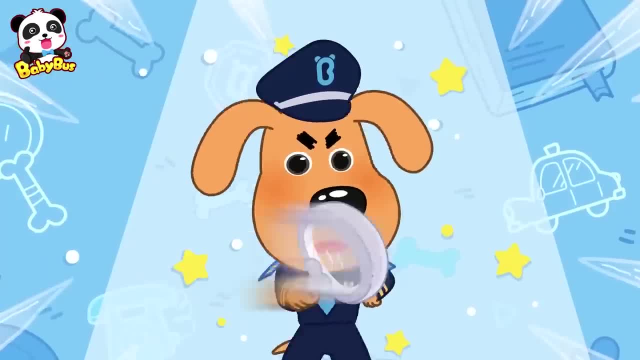 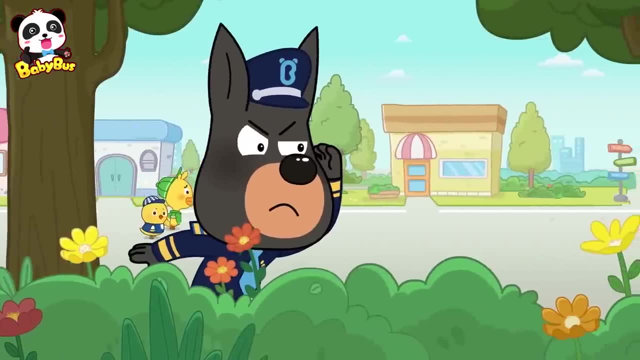 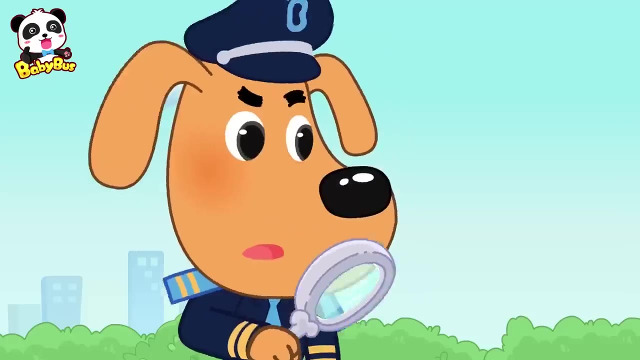 Right, There's no case that I can't solve. The footprints are only on the manhole covers. Hey kids, What game were you playing just now? Jumping on the manhole covers. It's so much fun. Stop Jumping on manhole covers can be very dangerous. 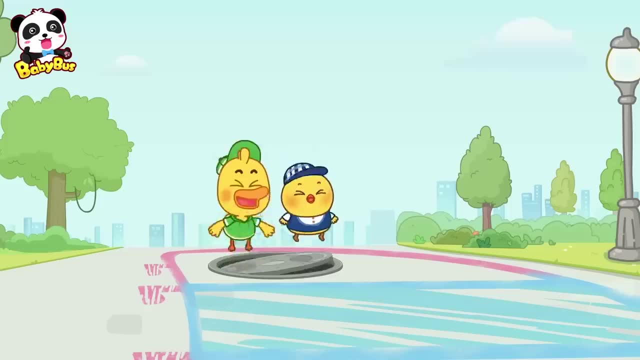 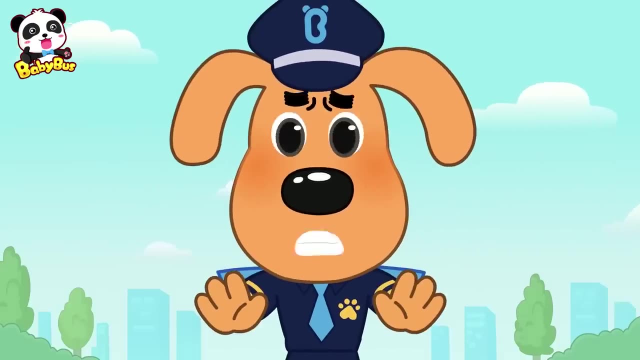 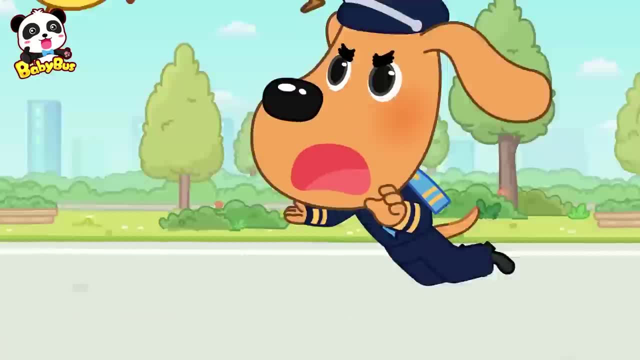 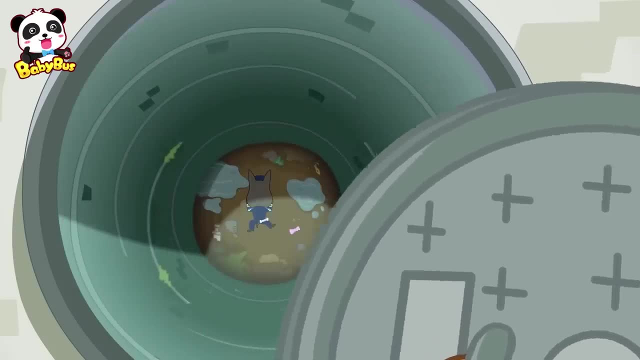 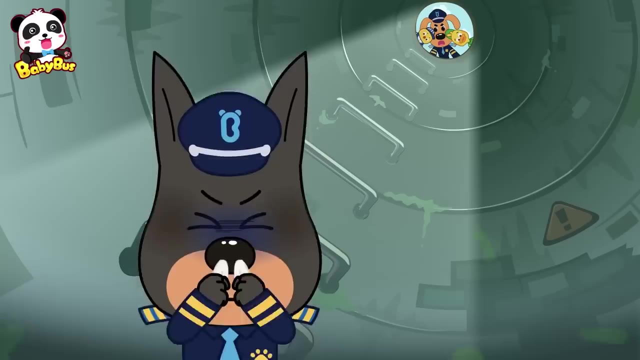 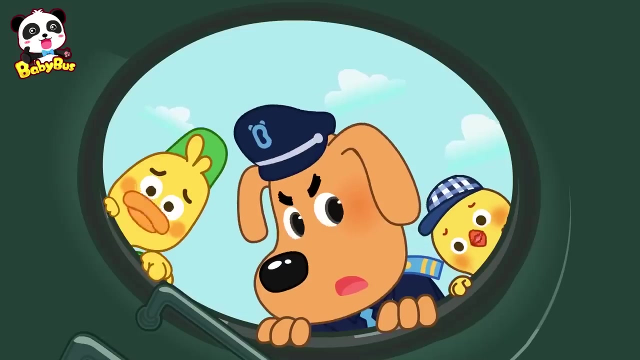 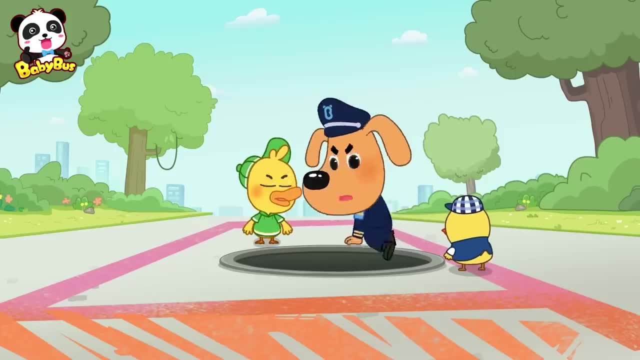 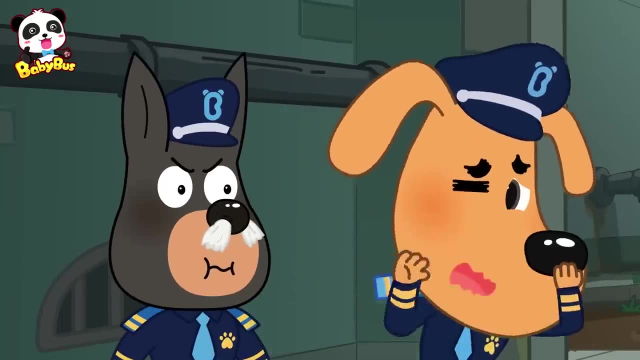 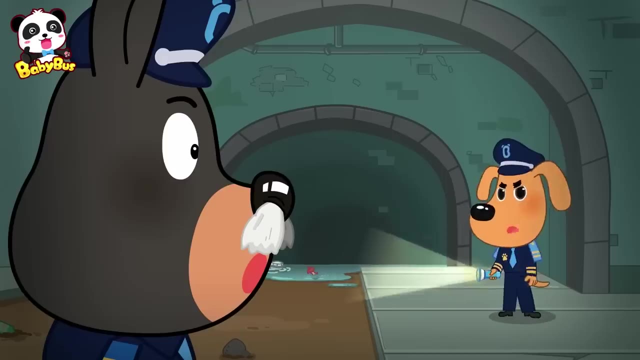 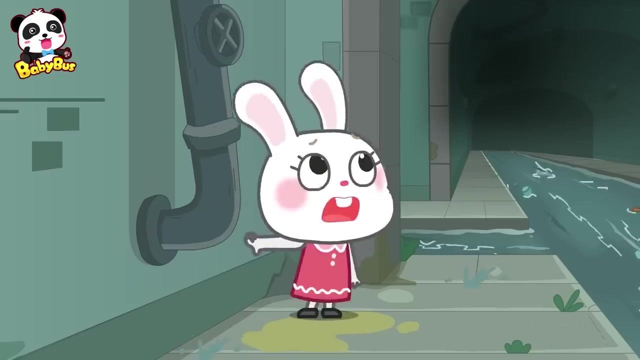 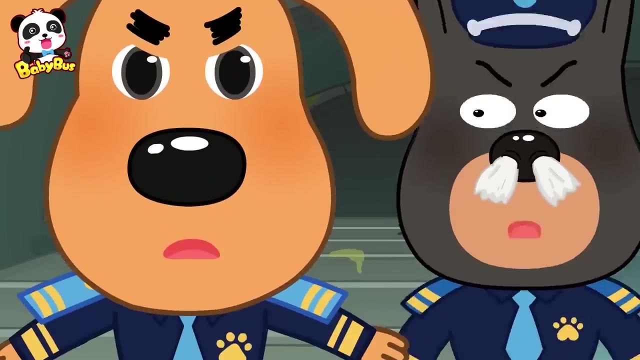 I'm going down to help Officer Doby find Little Rabbit. It's Stix down here, Stinks down here. This way's blocked Little Rabbit would have gone this way. Somebody help me please. The tunnel splits here. Which way should we go? 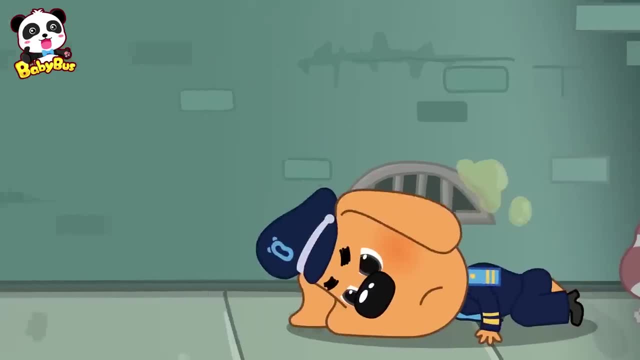 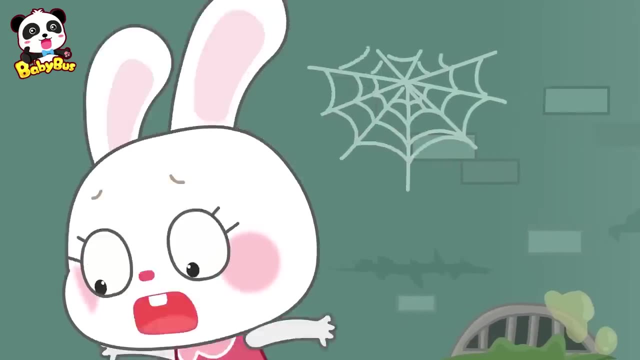 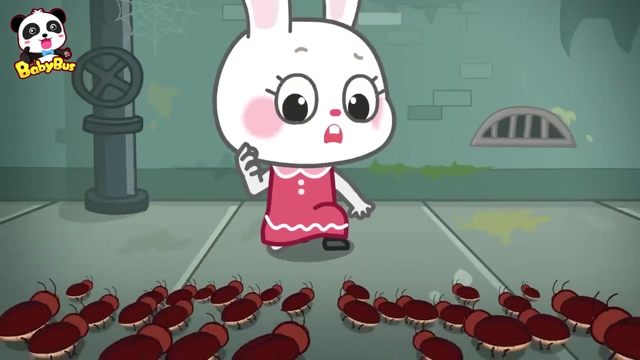 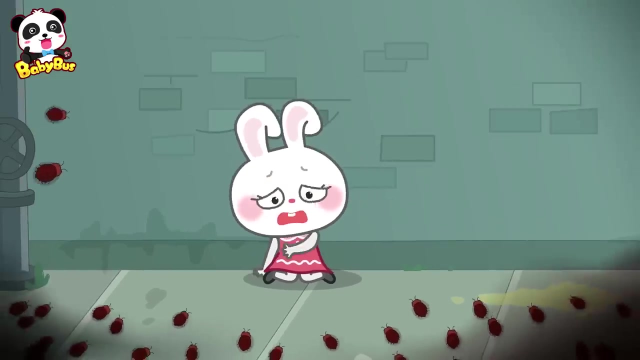 Let me listen, I'll go that way, Huh, OK, Oh, That way. No, Stay away from me, Little Rabbit. Uh, Oh, no, Oh Laa, Aaaa, The tunnel splits, Little Rabbit, That's it. 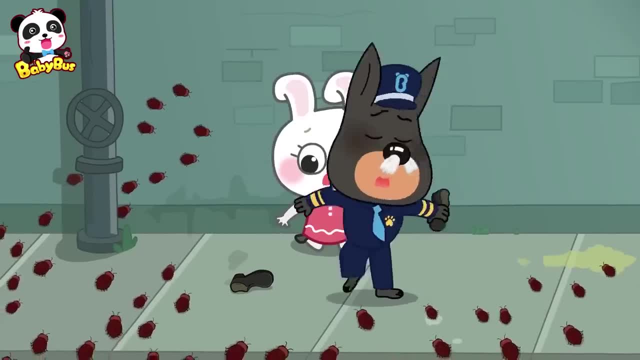 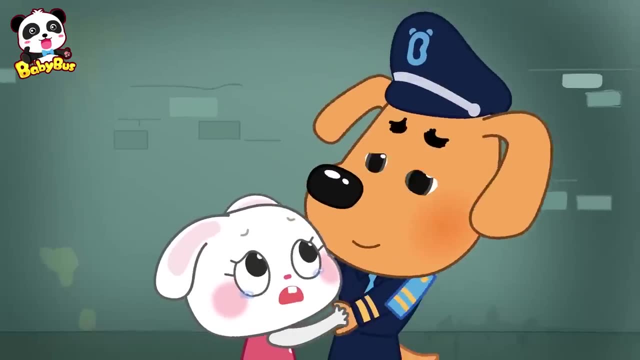 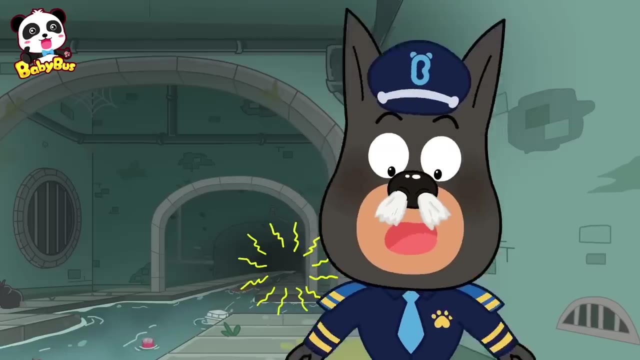 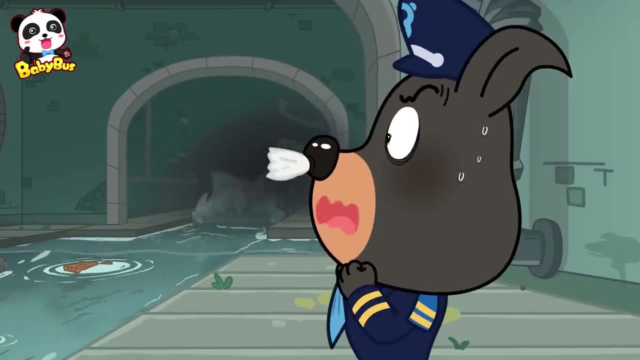 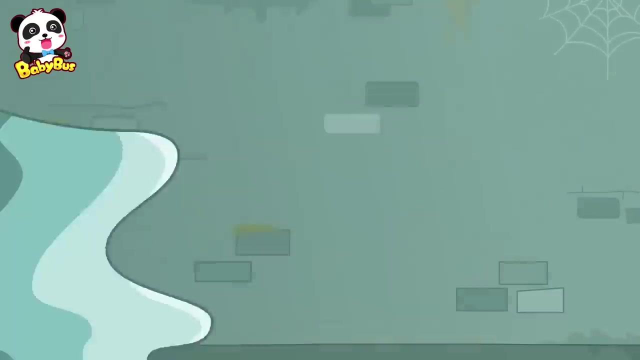 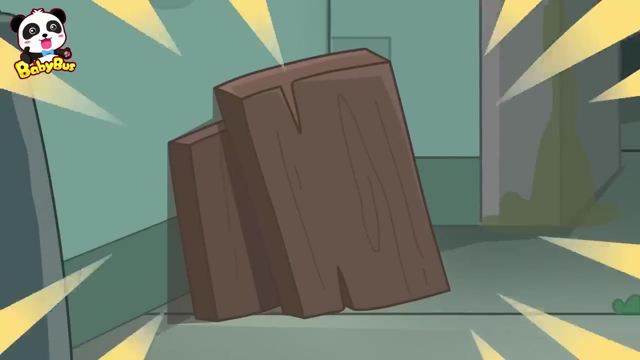 Ah, Ah, Go away. Go away, Sheriff Labrador. Don't worry, little rabbit, We'll get you out of here. Oh no, The wastewater is coming this way. Let's run. It's moving so fast. Toby, use those boards. 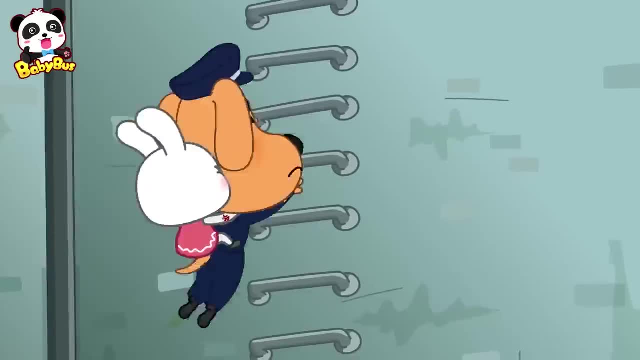 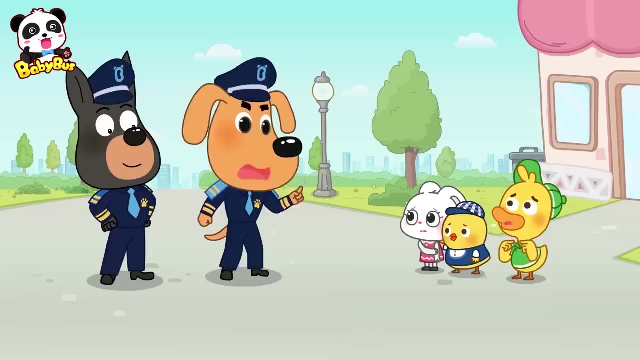 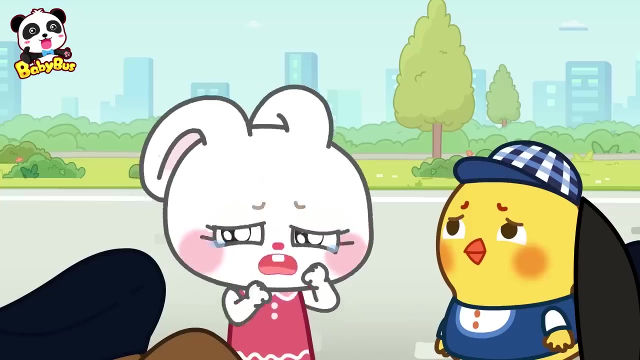 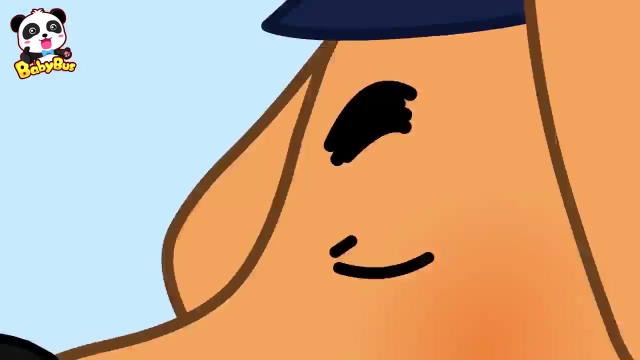 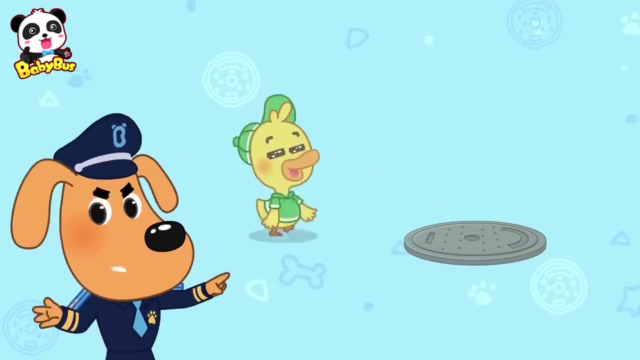 Chaka Kids remember: Never jump on manhole covers again. It can be very dangerous. It was so scary down there. We'll never do that again. Sheriff Labrador's Safety Top Kids. don't step on manhole covers on the street. 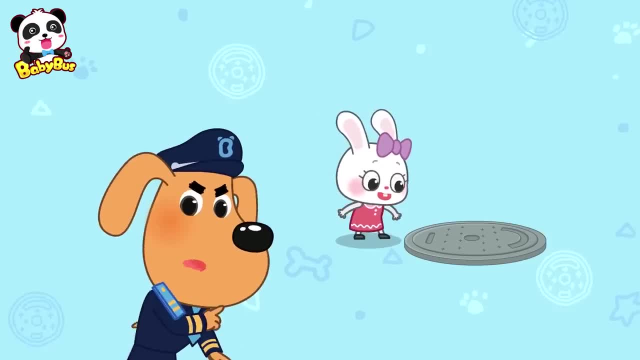 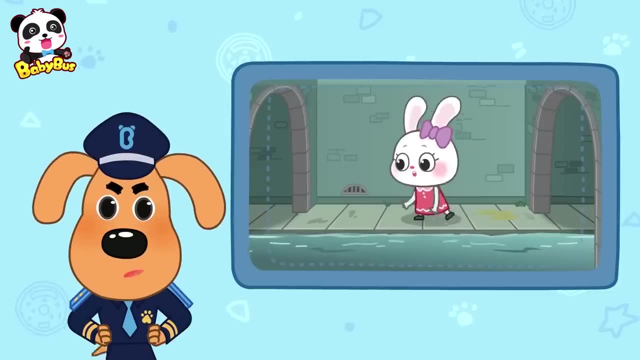 And keep away from them. when you walk. You might fall down and get hurt if you step on a broken or worn manhole cover. Also, the complicated sewer pipes, harmful gases, wastewater, cockroaches and mice under the manhole cover will make it hard for you to climb back out. 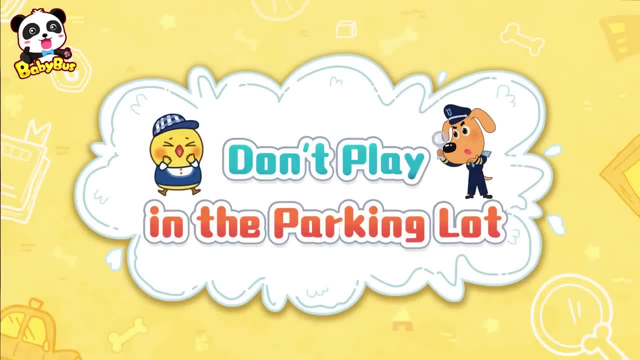 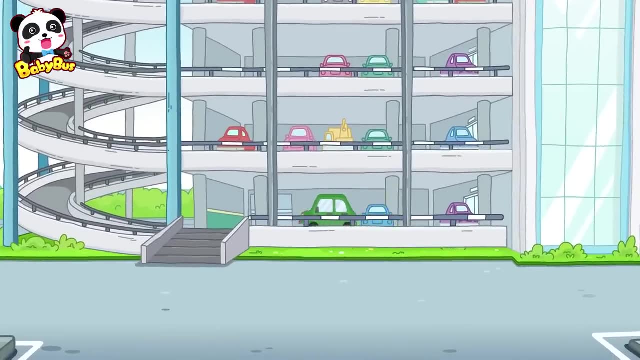 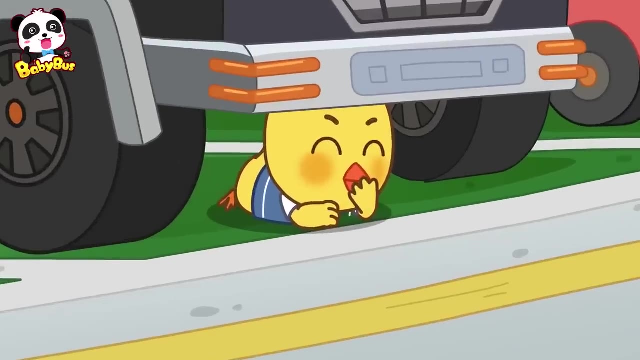 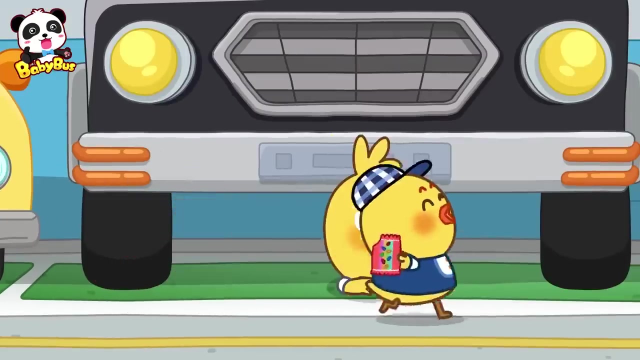 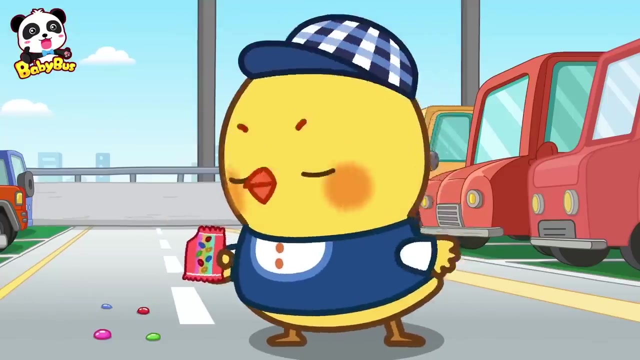 Woof, Don't play in the parking lot. Huh, Huh Ha. Haha, I found you, Uh-oh, Now it's my turn. Hahahaha, You'd better find a good place to hide. Huh, Huh. 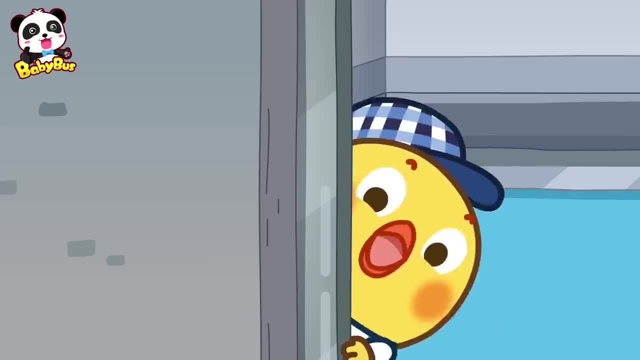 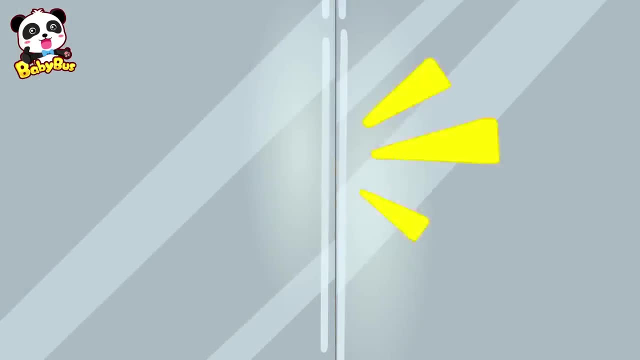 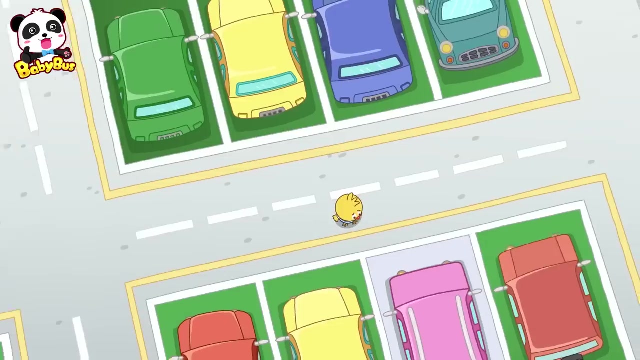 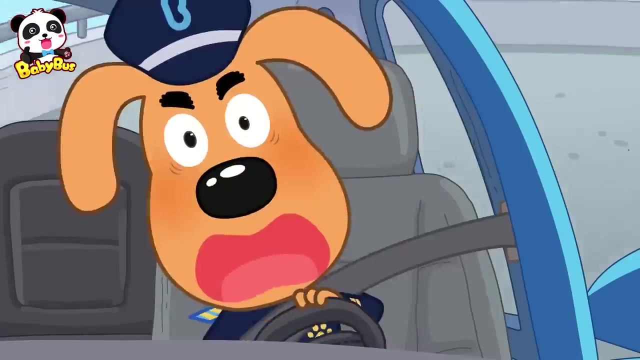 Ha, Huh, Hahahaha, Huh, Huh, Huh, Brother, Brother, Huh, Little chick, Little chick. where are you? Little chick, Little chick, Ah, Ah, Ah, Ah Ah. 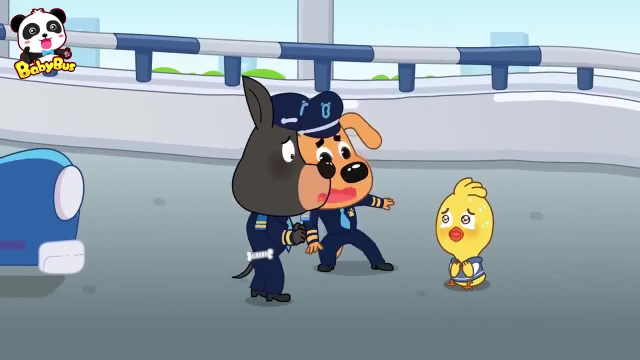 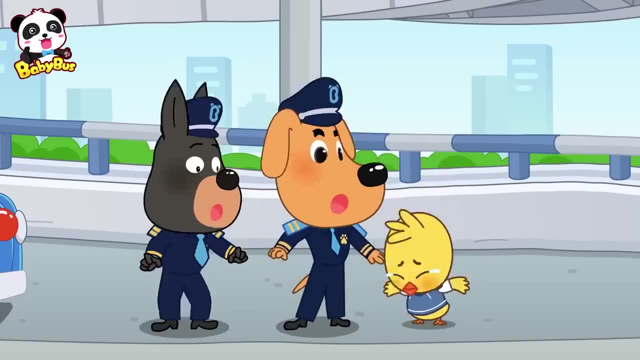 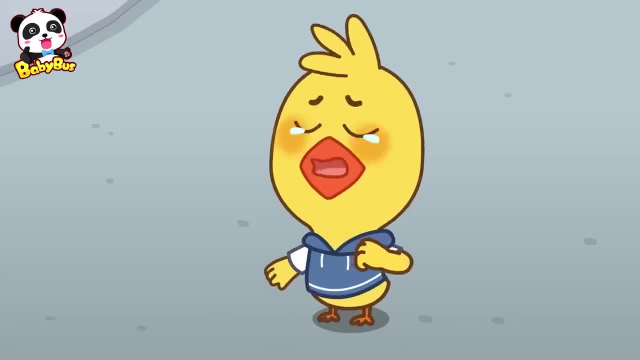 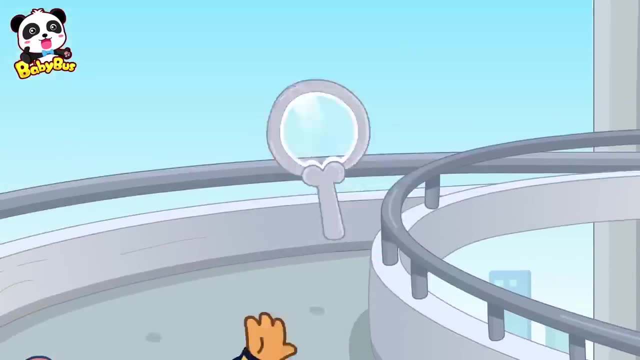 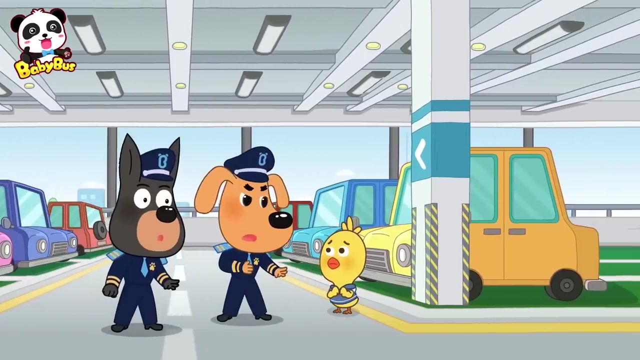 What You were playing hide-and-seek in the parking lot. That's really dangerous. Ugh, Please help me find my little brother. Don't worry, There's no case that I can't solve. Hey kid, Were you playing hide-and-seek on this floor? 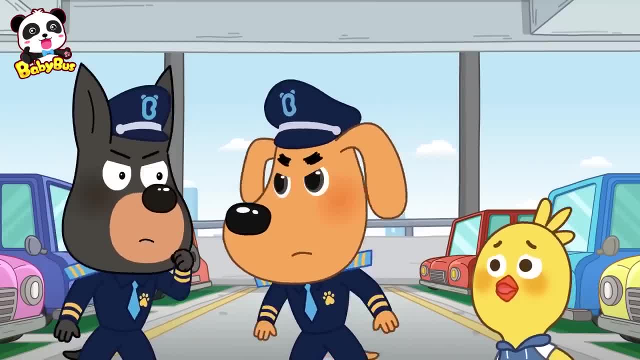 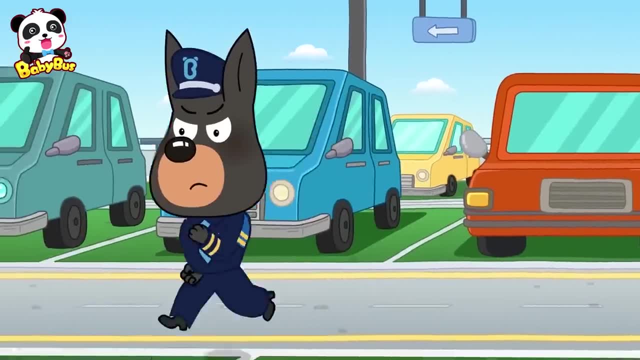 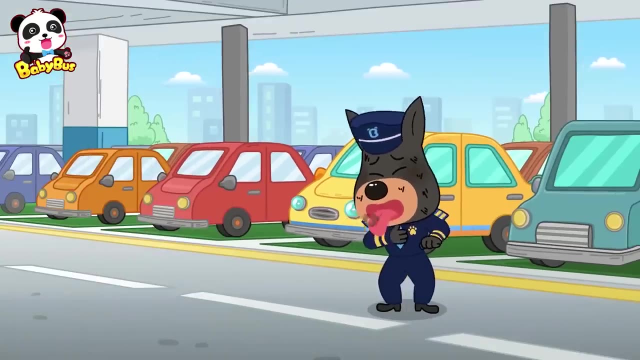 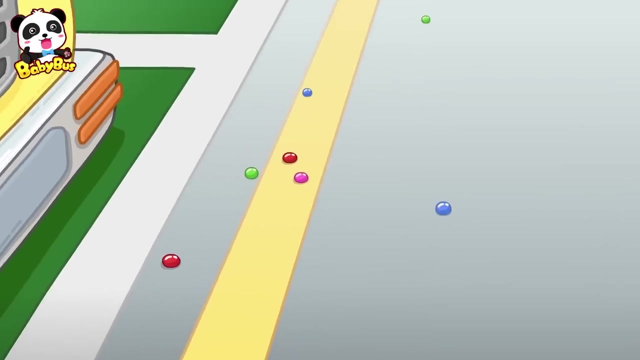 Uh-huh. We need to search every corner of this floor. Copy that: Ah Ah, Ah, Oh, Oh Oh. Little chick, Little chick, Huh, Ah, Ah, Little chick, Oh, Huh, Huh. 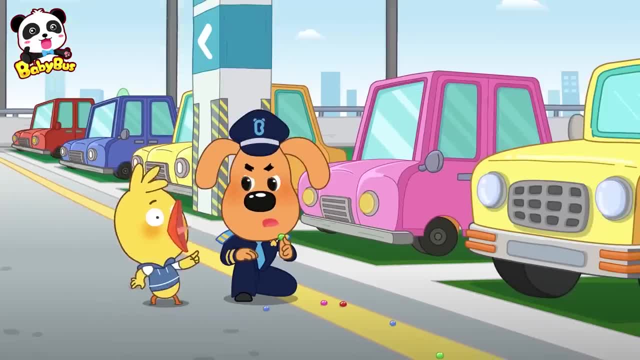 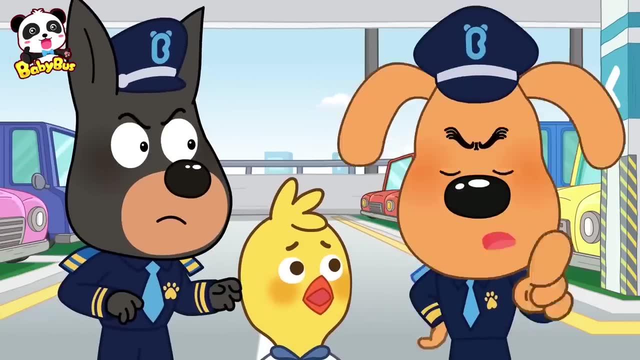 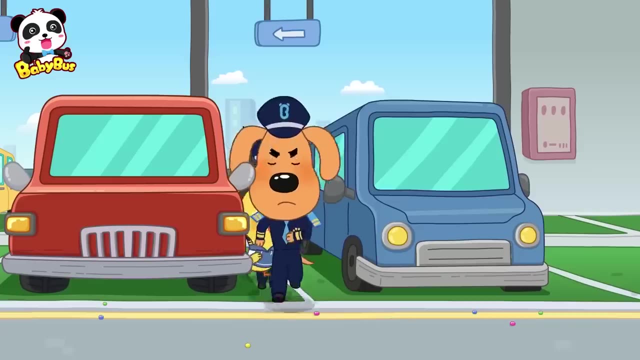 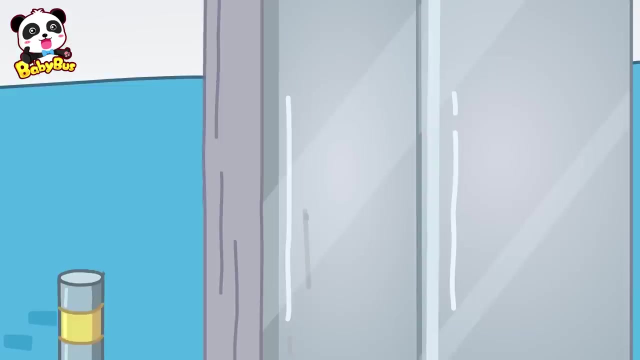 Oh, Oh, Huh. Ah, These are my little brother's jelly beans. Huh. Hmm, little chick might be around here somewhere, then We might find him by following these jelly beans. Huh, The jelly beans have stopped here. 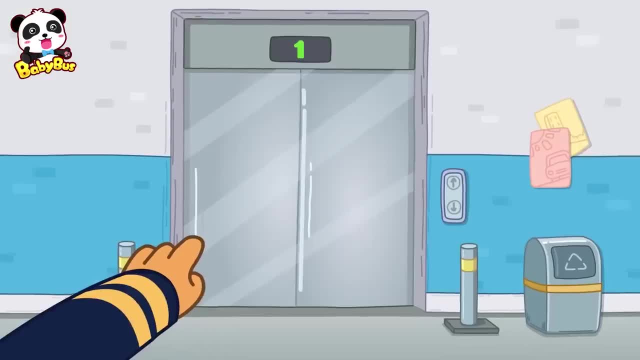 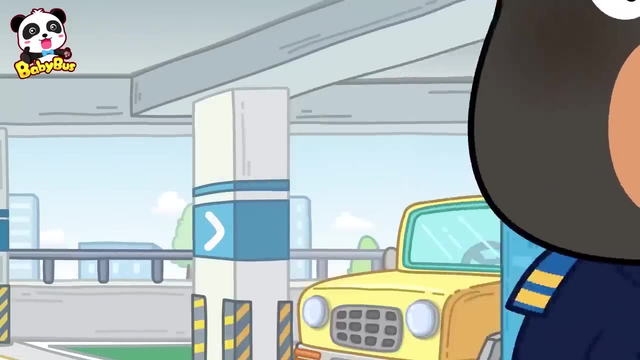 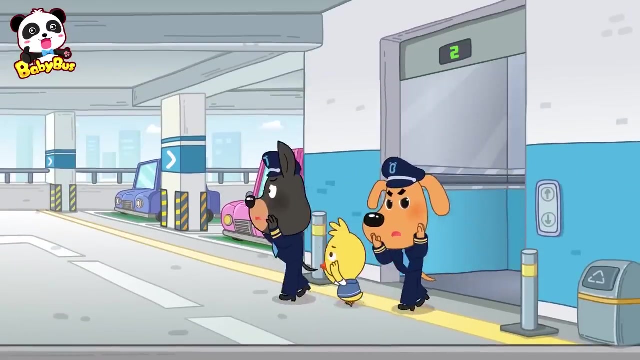 That means… Little chick might have taken the elevator. It's dangerous around here. We need to find him as soon as possible. The second floor: Little chick, Little chick. Excuse me, have you seen a little chick this tall? No, I haven't. 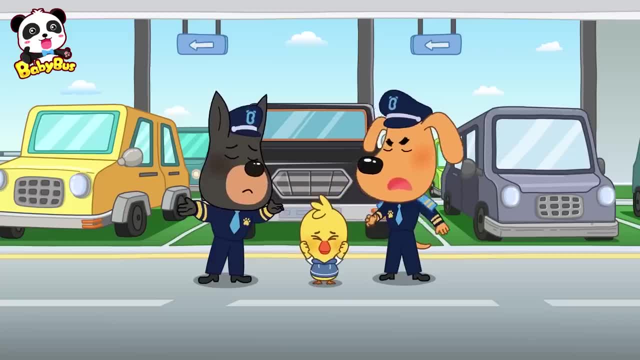 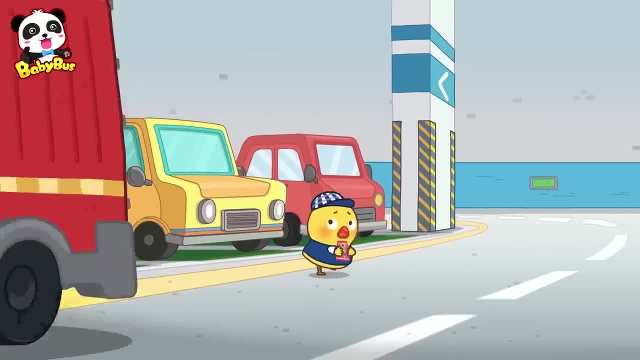 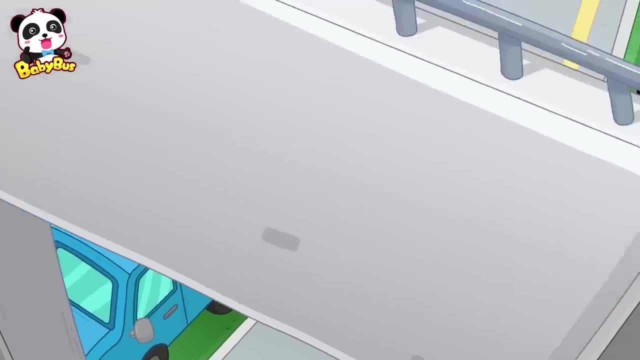 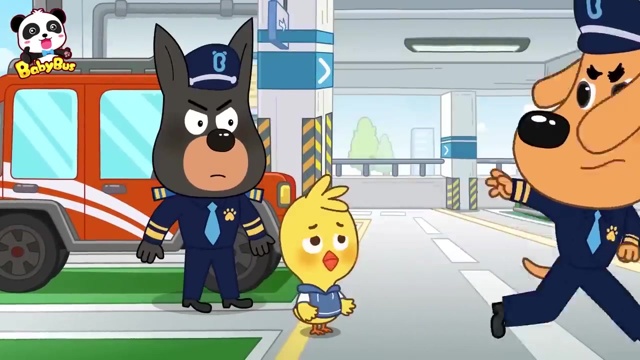 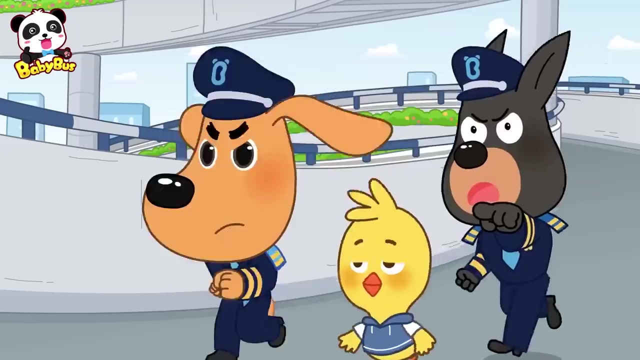 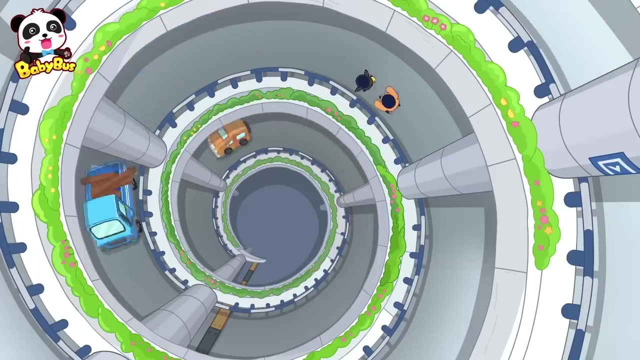 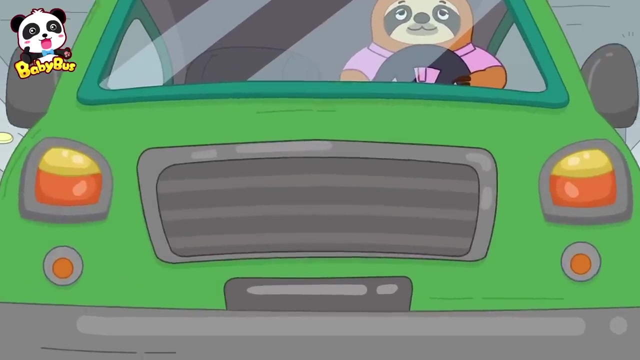 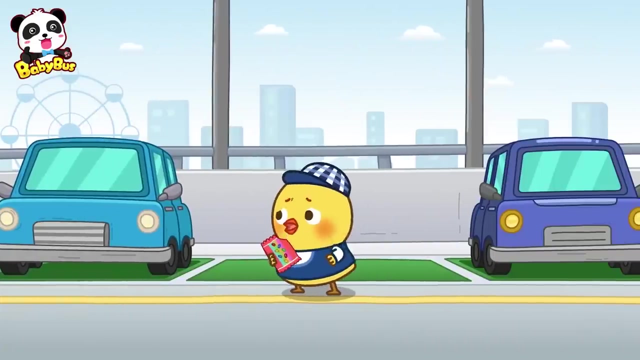 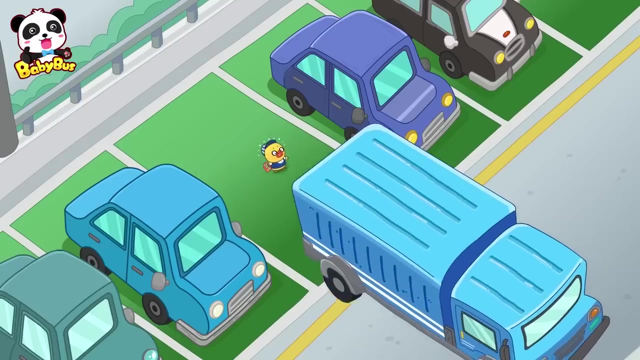 Toby found anything. No, Oh, my little brother. Brother, wait, Where are you, Brother, It's little chick. Brother, Brother, It's from up there. Follow me, Little chick, Little chick, Watch out, Help. 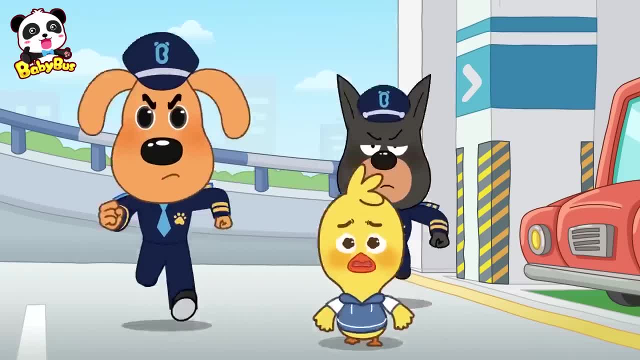 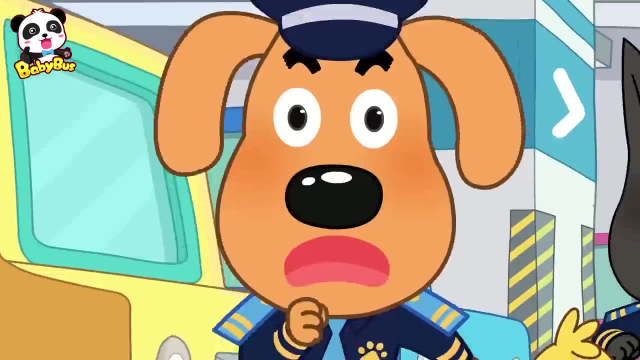 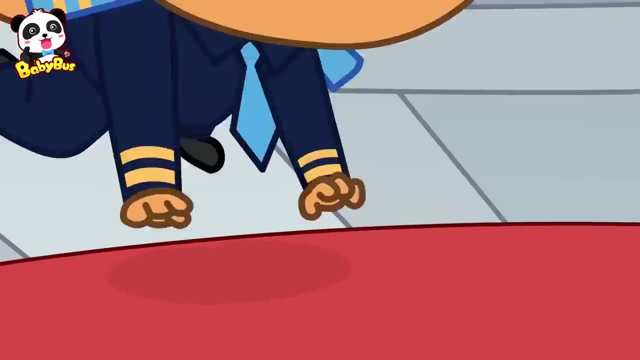 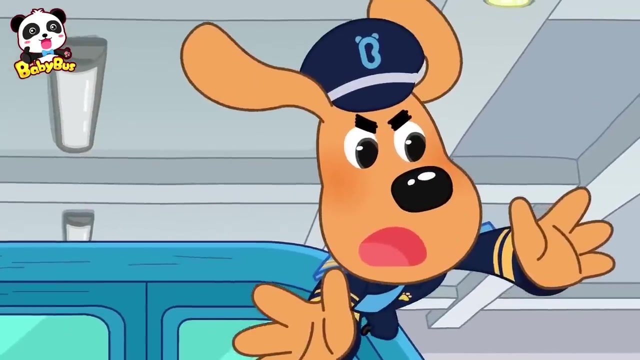 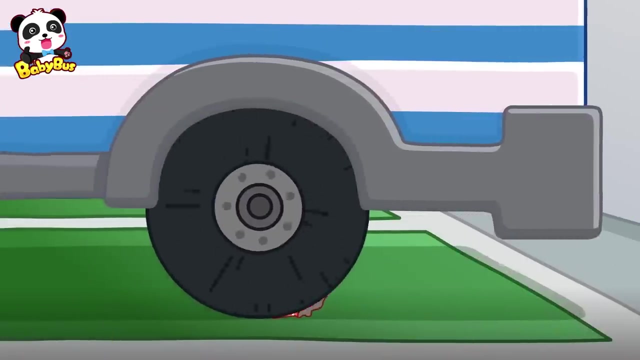 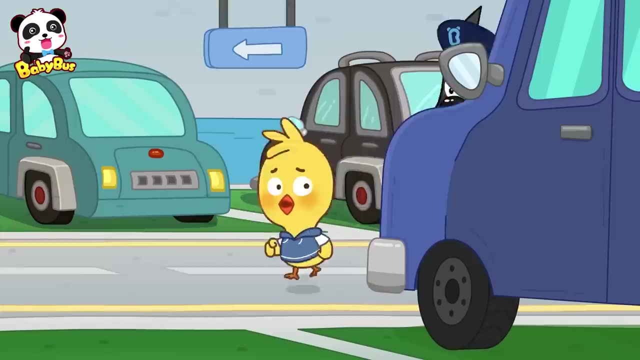 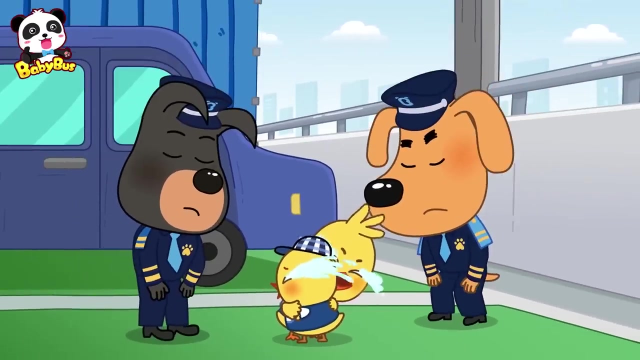 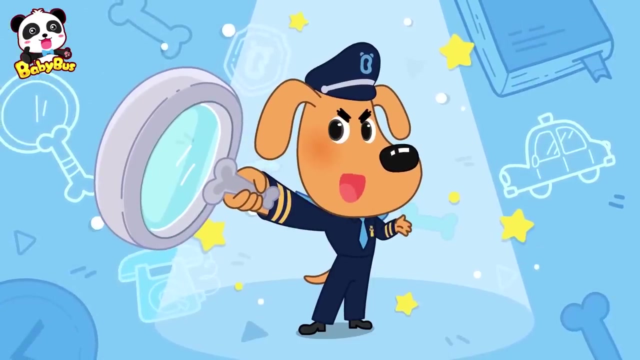 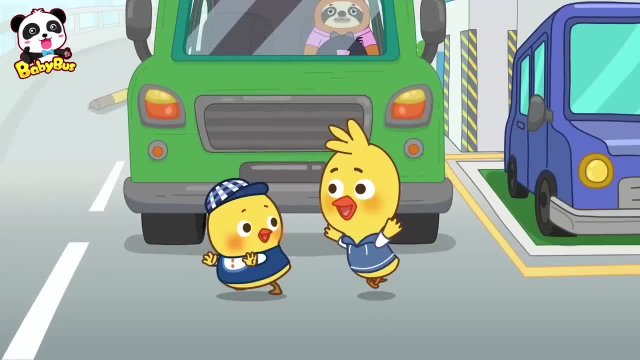 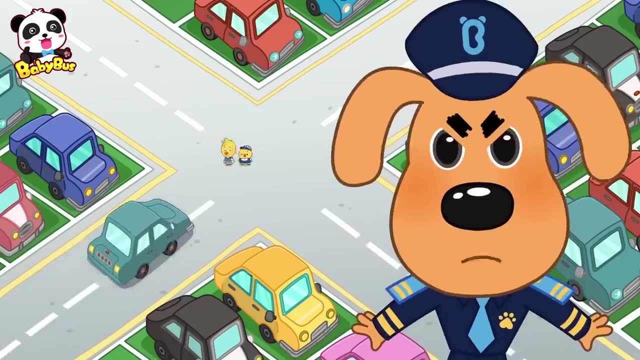 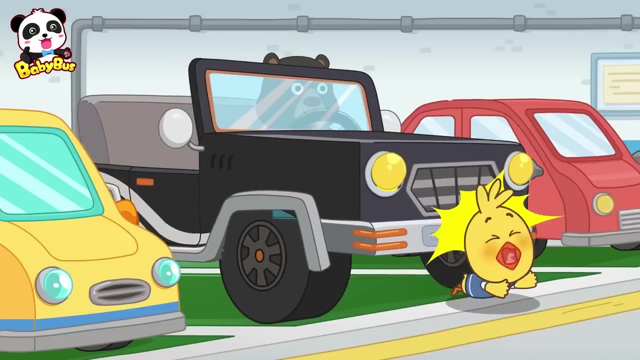 You might be in a car's blind spot As you're not tall enough to be seen by the driver, And with so many intersections in a parking lot, drivers can't always react immediately and accidents could happen. Also, beware of idle cars, as you could easily get hurt if they start to move. 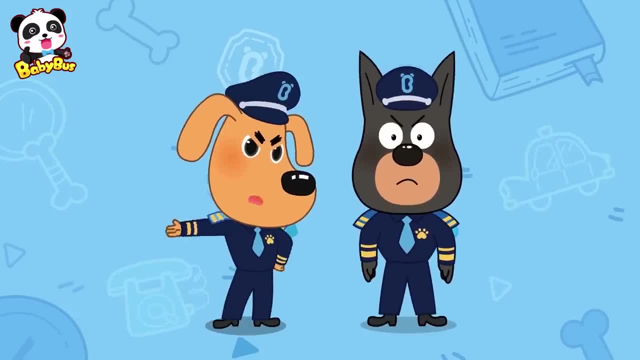 Remember to stay alert when you're in a parking lot and don't play around. Always safety first.